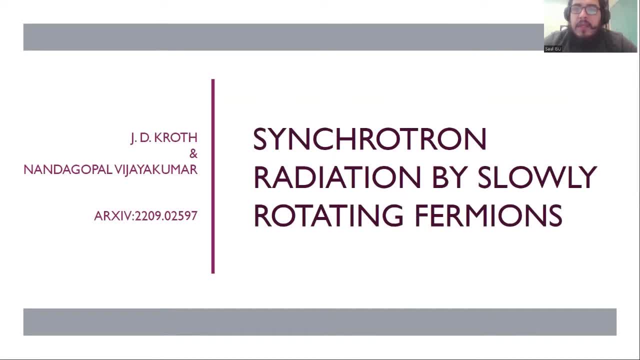 by JD Kraut and Danda Gopal. They will talk about the synchrotron radiation by the slowly rotating fermions. This talk will be given by both speakers. Danda Gopal will first introduce the essentials for the synchrotron radiation and then JD will tell us about 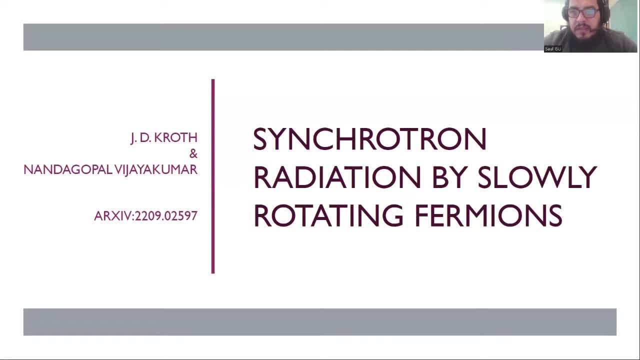 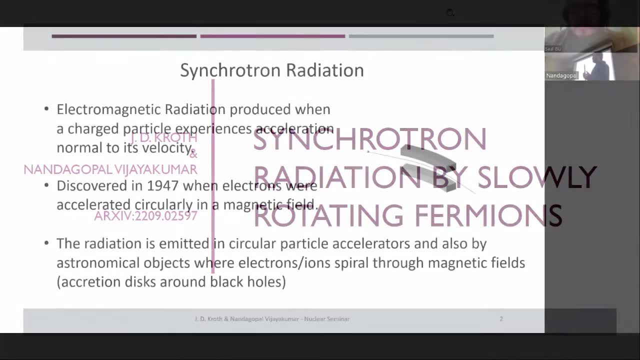 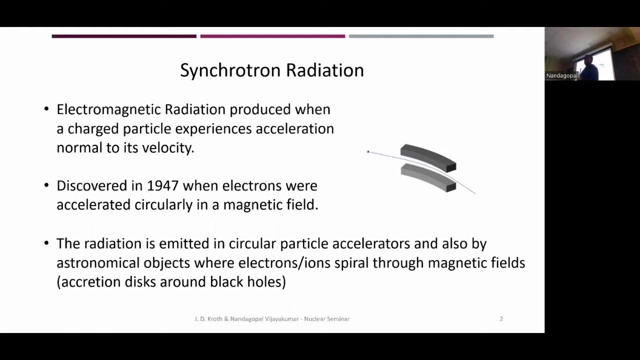 the numerical results. Let's just hear from them. Thank you again and apologize for the technical problems. Whenever a charged particle undergoes a curved path, it produces this type of radiation, And the best way to make a charged particle go through a curved trajectory is to apply 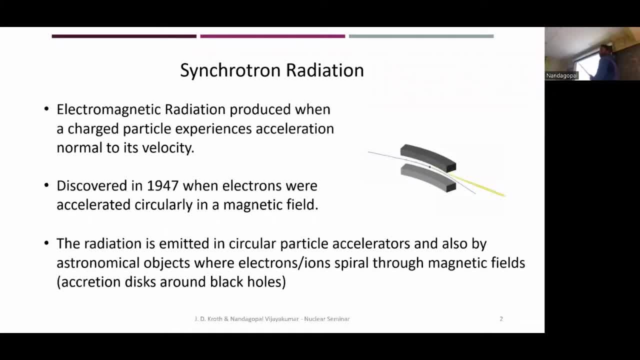 a magnetic field. In fact, this was how synchrotron radiation was discovered, when high energy electrons were accelerated by a magnetic field inside a circular particle accelerator. So in experiments inside circular accelerators it is important to consider the synchrotron 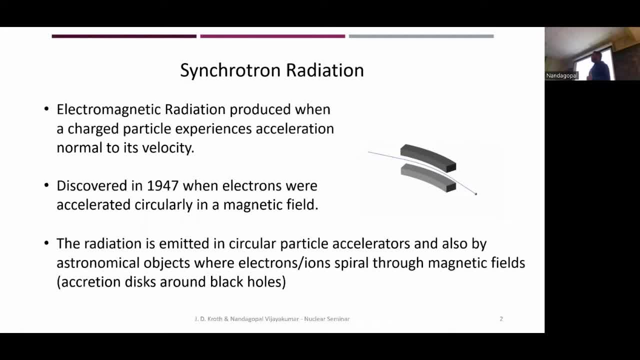 radiation losses. Synchrotron radiation also occurs in several natural phenomena, like in accretion disks around black holes, where we have charged particles like electrons or ions which are spiraling inside a magnetic field. The variables are also speculated to be a source of synchrotron radiation. 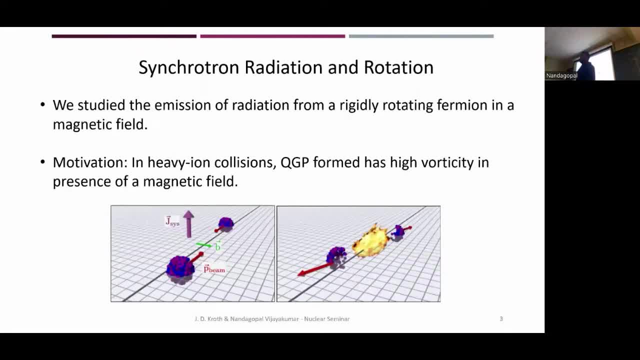 Now coming to our work. we studied the synchrotron emission from a charged fermion which is undergoing rotation, placed in a magnetic field. Now, magnetic field itself imposes a rotation on the charged particle, but here we are imposing an independent, rigid rotation. 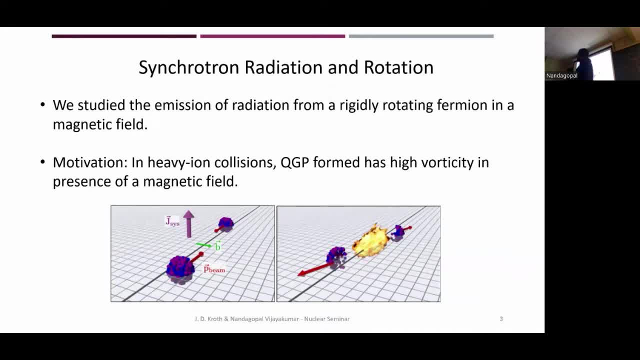 on the fermion. So the motivation behind this comes from relativistic, heavier and co-efficient radiation. Now, if the magnetic field itself imposes a rotation on the charged particle, heavy ion collisions where we have two nuclei are bombarded against each other, which results. 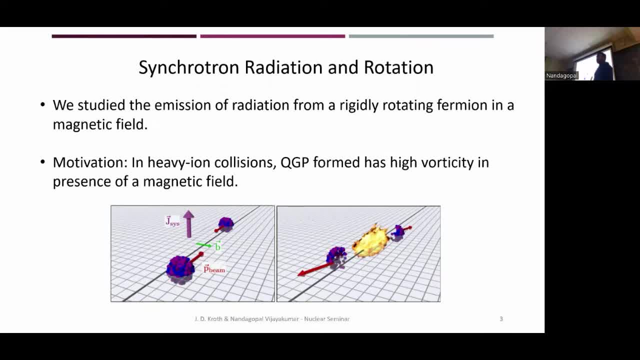 in the production of quark-blown plasma. Inside this quark-blown plasma we have fermions which are in very strong electromagnetic fields. Now if you look at this figure, you can see that the two nuclei collide against each other with an impact variety, and this results in. 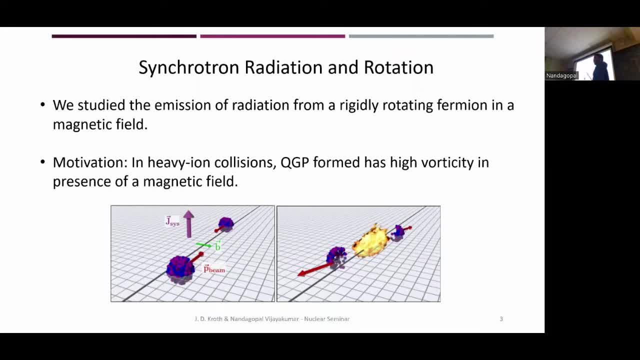 the quark-blown plasma to have non-zero angular momentum when the collision happens, and this Hof-Center collision happens, And this is the reason for the high vorticity of the plasma Now. so there is rotation from the magnetic field as well as the rotation of the medium. 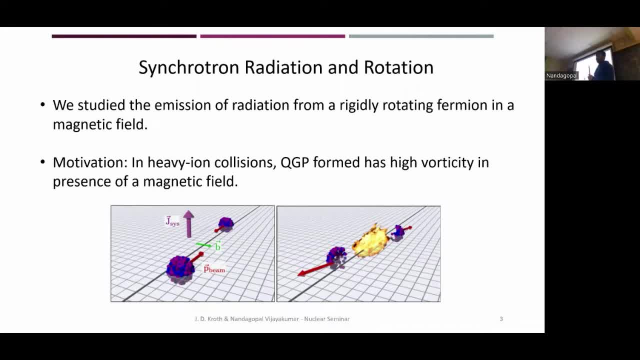 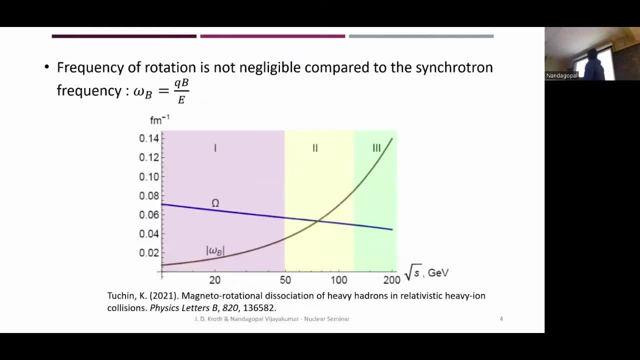 The charged particle is in magnetic field in rotating medium, So the rotation due to the medium is not negligible. So compared to the synchrotron frequency. That's why we are specifically studying the effective rotation in synchrotron radiation, As we can see from this figure, which was 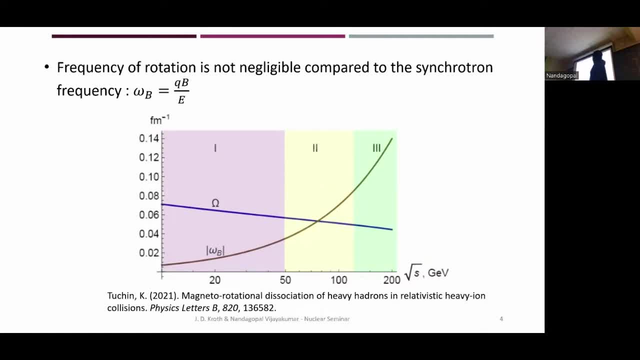 obtained by Dr Tuchin. in the following paper we can see the vorticity of the quark-blown plasma represented by capital. Omega is compared with the synchrotron frequency. Omega B is given by the following formula: 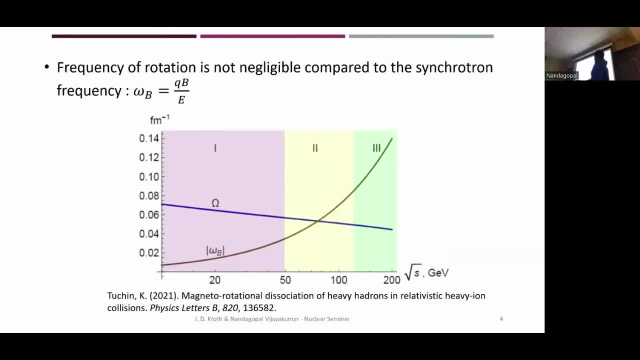 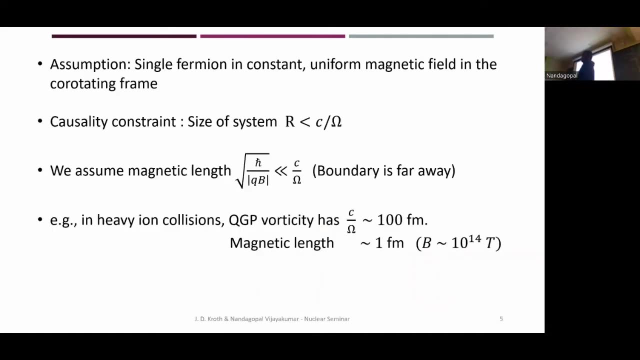 And if we can see that the vorticity is not negligible compared to the frequency or frequency created by the magnetic field. Now in our work we did a simplified model where we just take a single fermion and we assume that in the correlating frame of the fermion the magnetic field is constant and 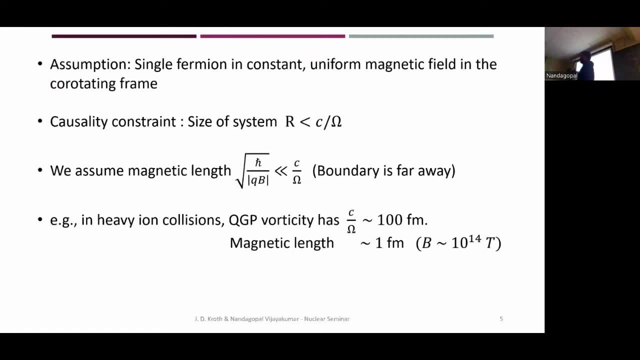 uniform. So it's a much more simplified version than what happens inside a QGP, And that's so just to make the calculation easier as a first step. Now, when it comes to rotating relativistic system, there's a causality constraint To. 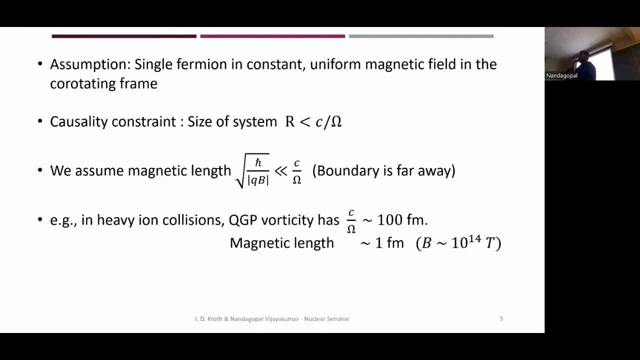 understand this causality constraint, we need to look at the speed of a particle with undergoing rotation, So which is given by the rotational frequency. Then there is also the speed of the particle with its undergoing rotation, which is given by the rotational frequency, And then there is the speed of the particle which is going. 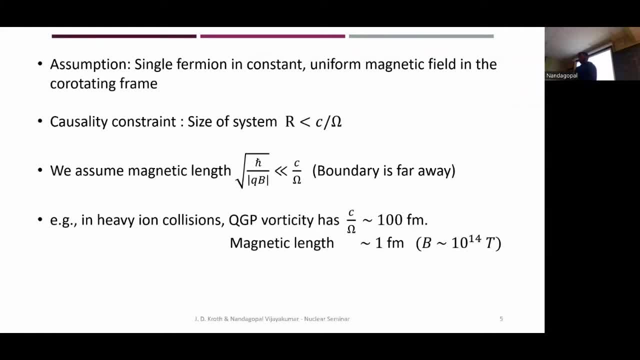 frequency times, the radian distance of the particle. So the speed of a particle increases linearly with the distance from the rotation axis. So at one point that speed can cross the speed of light, which can happen. So this imposes a maximum allowed distance. 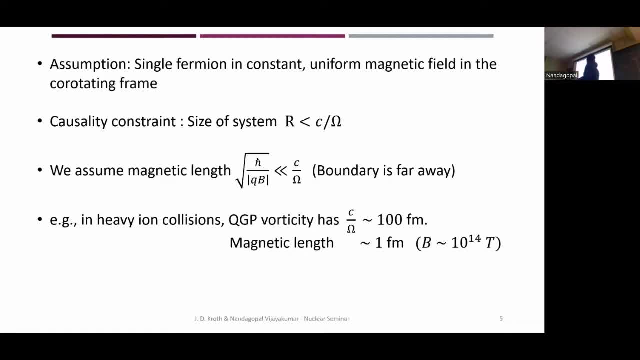 for rotating systems, radian distance for the radian systems, And this is simply given by plugging in C for the velocity of the particle. So we cannot have the size of the rotating system to exceed this causal boundary of C over omega. Let's look at C over omega. 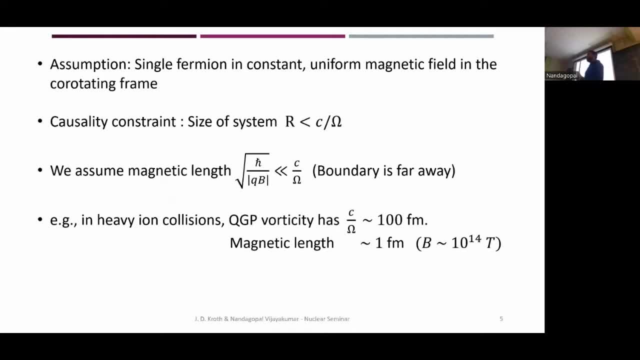 Now, quantum mechanically, what this means is that our wave function. we should set boundary conditions such that the wave function vanish at the C over omega. But that is difficult to do for a direct spinner. possible but difficult. But in this calculation we'll use a different. 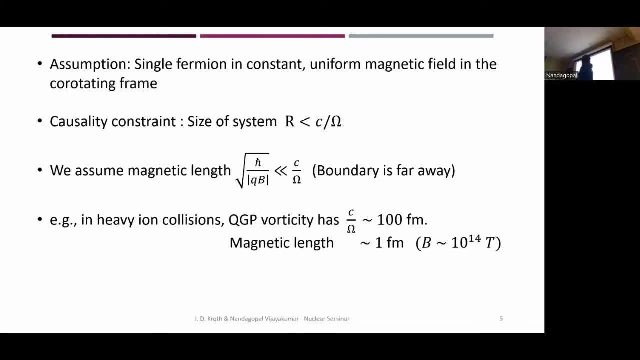 assumption, which is that the magnetic length given by the formula shown here is the characteristic length beyond which the wave function is suppressed in a magnetic field. So this magnetic length we will take to be much smaller than the size of the causal boundary, And so this technically means: 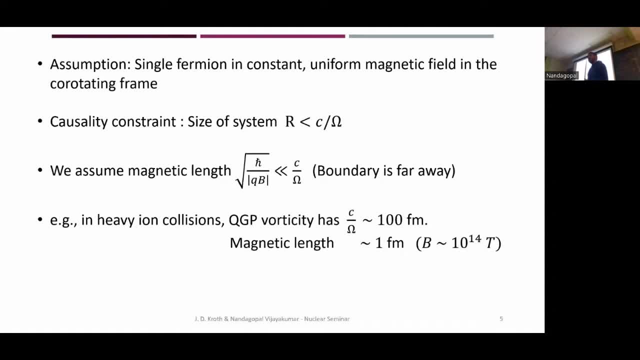 that the boundary is very far away, So we can take the wave function to vanish it at large, larger distance or infinity, instead of imposing it to vanish at one specific point. To see whether that this assumption makes sense, we'll get, we'll plug in some numbers. 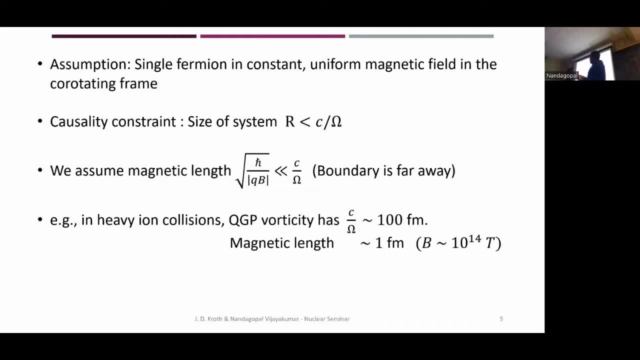 So in QGP the vorticity corresponds to size of the grade, the causal boundary to be about a hundred Fermi's, which is not very big, but the magnetic field achieved in these in heavy and collisions, are so huge that the magnetic field 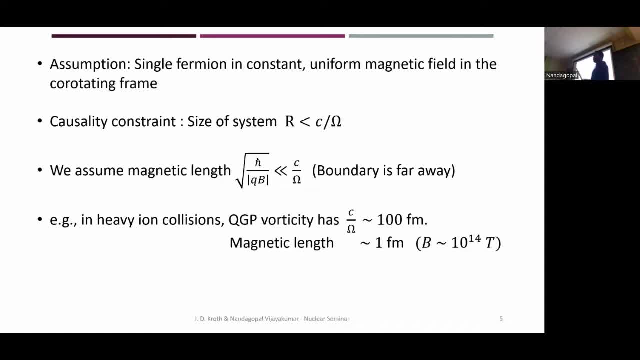 achieved in these in heavy and collisions are so huge that the magnetic field achieved in these in heavy and collisions are so huge- about 10 to the four of the order of 10 to the 14 Tesla's- that the magnetic length is even smaller. 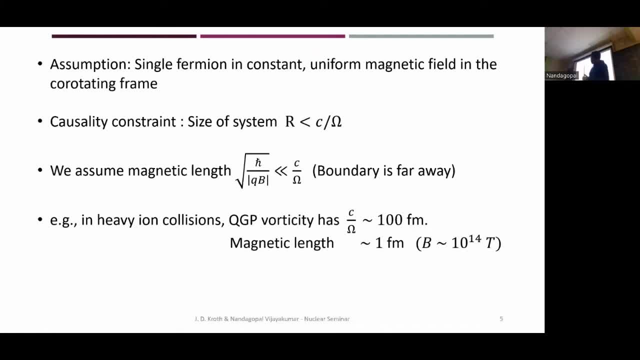 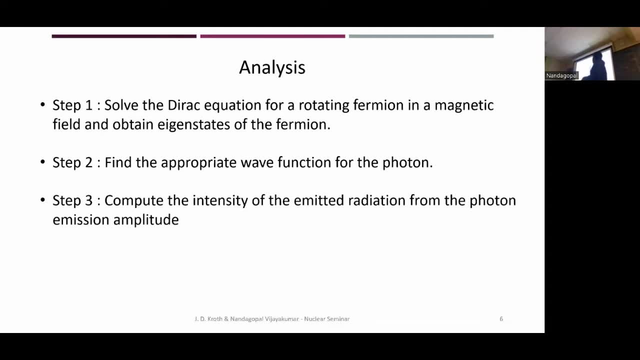 of the order of only a firm, So this assumption makes sense. Now our analytical procedure can be broken down into three steps. First, we solve the direct equation for a rotating fermion placed in the magnetic field, And we obtained the energy spectrum and the eigenstates. 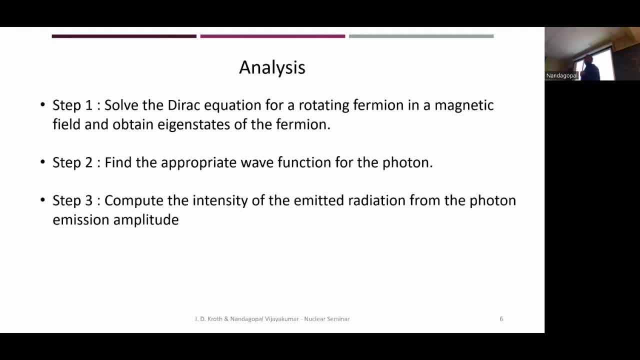 Second step is straightforward: to find the wave function of the photon in the cylindrical coordinates. We'll be using cylindrical coordinates because that's the most convenient one to impose rotation. And the final step is: once we get these wave functions, we can calculate the amplitude of photon emission. 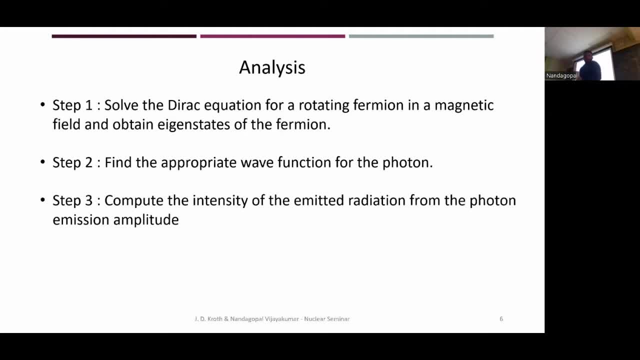 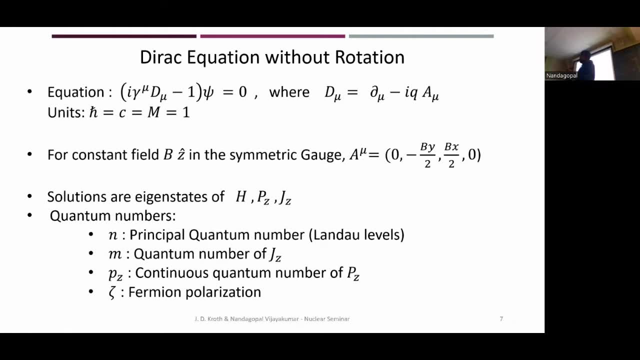 And from that the total radiation density. Okay, so let's dive right into the first step, Which is the solved direct equation. But before we go to the direct equation with rotation, we switch off the rotation and see what the solution looks like. 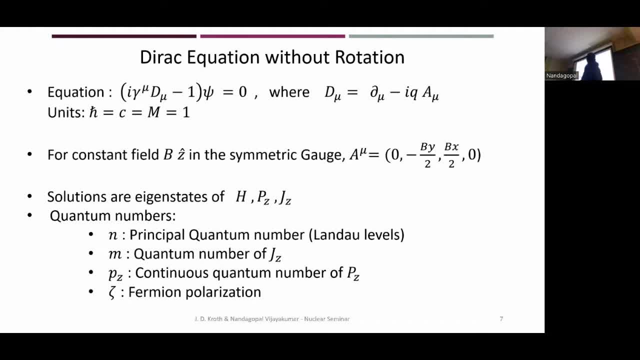 So in this case the direct equation is modified by: the: ate is the usual derivative plus the for vector. And also one more thing: we'll be working in units where X equals and C equals one and capital M, which is the mass of the firmium, is also set to. 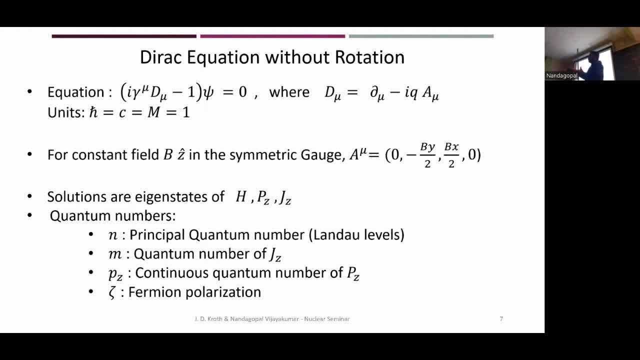 we will be working, Dimensions will assume that the magnetic field is along the sea head direction and in the symmetry. that will give us the following quality potential: And this gives us and solutions are island states of the Hamiltonian, the C component of linear momentum and the C component of the total angular momentum. 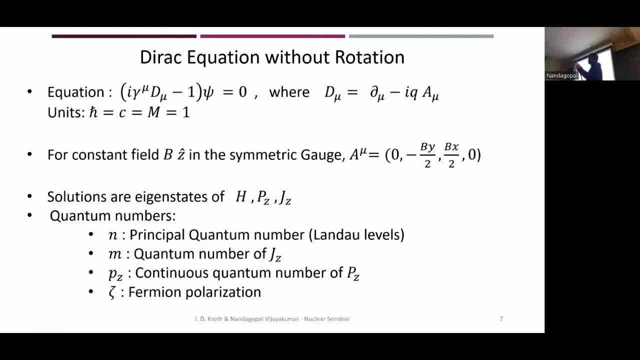 So this gives us the relativistic Landau states and our levels and check act twice by the following quantum numbers: the principal quantum number n, the angular number m and the continuous quantum number for PC. we also have Zeta, which characterizes the fermion polarization. 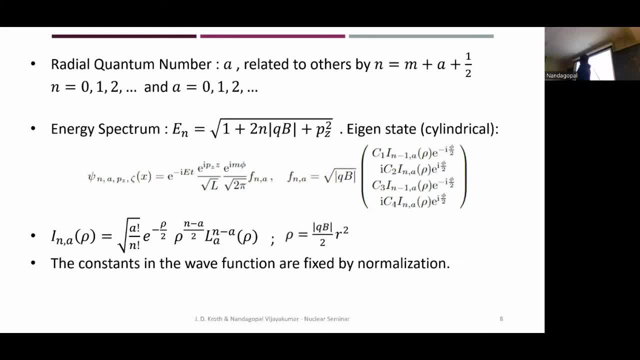 And now there is one more quantum number, radio number a, Which is not independent of the others. it depends on n and m, as shown in the relation. as shown, and we'll be working with n and a as the quantum numbers instead of n and m, because n and a are. 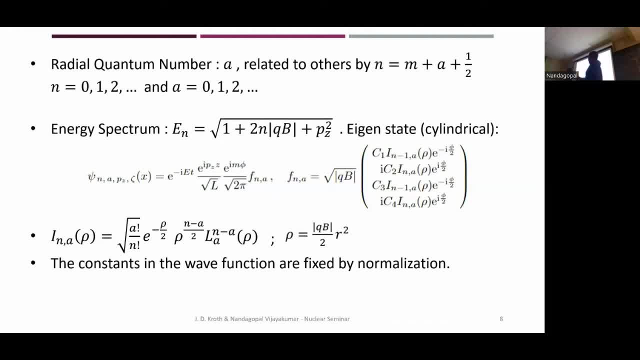 Non negative integers. so it's much more convenient to work with n and a, And the energy spectrum for In this case is given as follows, and we can see that the energy does only depends on On n and not on m, so there's a B2C- m. 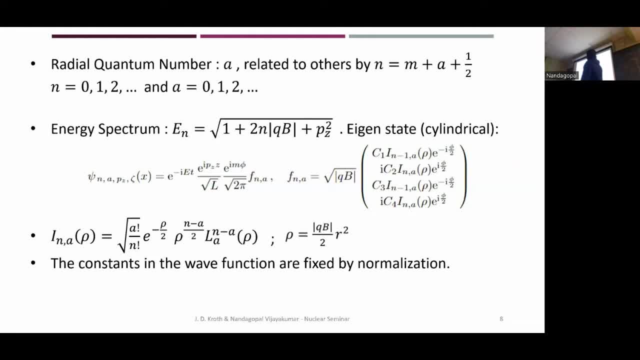 And the eigenstates are given by the following: a by spinner, and we can see that in this by spinner there is this function, this I function and I function consists of an exponential factor, a power law and the generalized laguerre polynomial. And we can see that the exponential factor makes, make sure that the wave function manage. 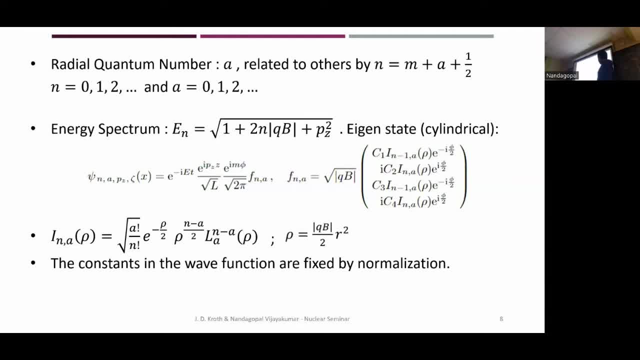 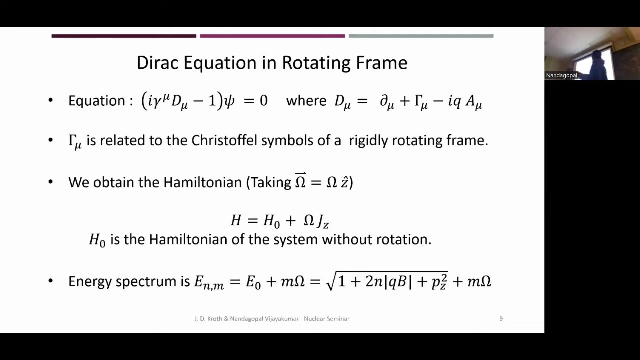 Off at large enough distance and in fact the characteristic length scale of that decay is indeed the magnetic length that we've seen earlier. The constants of the wave function are fixed by normalization. Now, coming into the rotating frame, the only difference that rotation brings is in the covariant derivative, is that it adds this term: gamma, mu term. 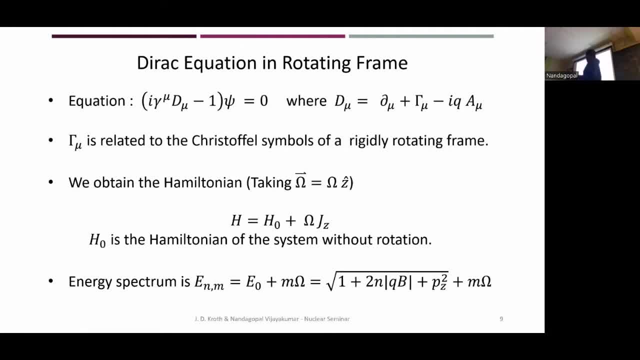 Which is related to the Christoffel symbols of this non-initial frame. What this does in the end is to introduce an additional term. in the previous Hamiltonian he writes now this: the Hampton without rotation. This additional term will be omega dot j will take the rotation vector to be along the z axis, along the axis of the magnetic field, and that gives us omega jc. 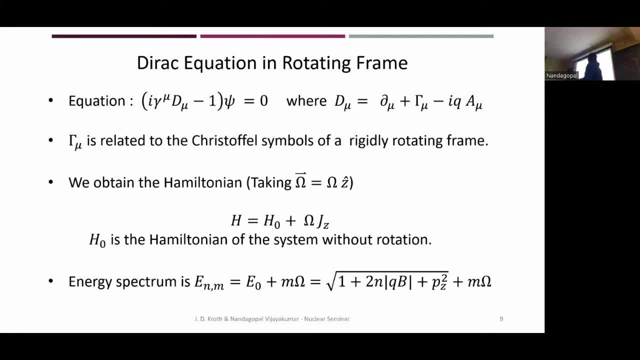 So, surprisingly, we, despite The Dirac equation and All the quantum mechanical approach, we have Rotation. the effective rotation is just the same as in classical mechanics. and So and we have seen that the eigenstate of H naught are also eigenstates of jc, so we can use the same eigenstates as before in this case. 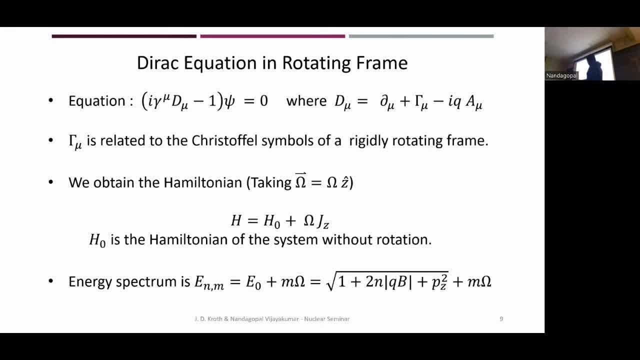 And So the only effect is to change the energy spectrum. this term is similar to Siemens splitting in hydrogen atom, So what it does is just lift the degeneracy or m with this idea. so the energy spectrum is shifted by this term m, omega. 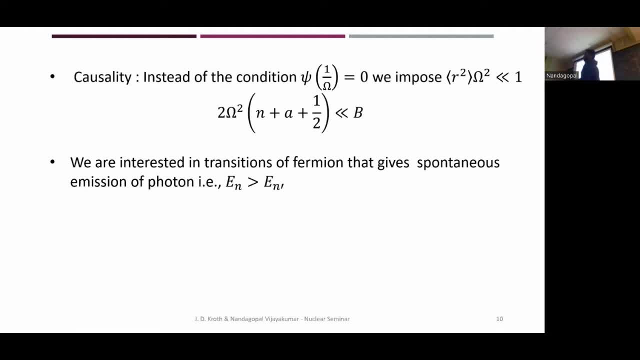 And We talked about the causality constraint. so, rather than use, impose the boundary condition that sigh vanish at one hour, Omega will impose the condition that The expectation value of the radial distance of the wave function square of the radial distance of the wave function. 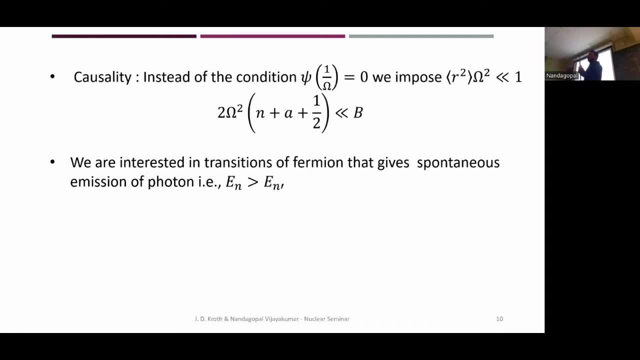 Is much less than the square of the size of the fossil model and that gives us the following: any quality. so as long as we are in slow rotation domain, Omega being respond be our Omega squared will be sufficiently large that we can use reasonable values for m and a. they are allowed. 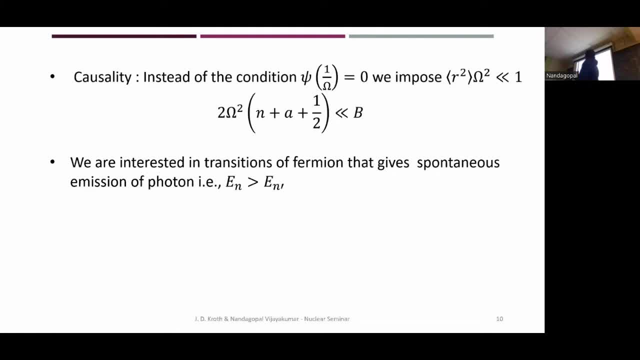 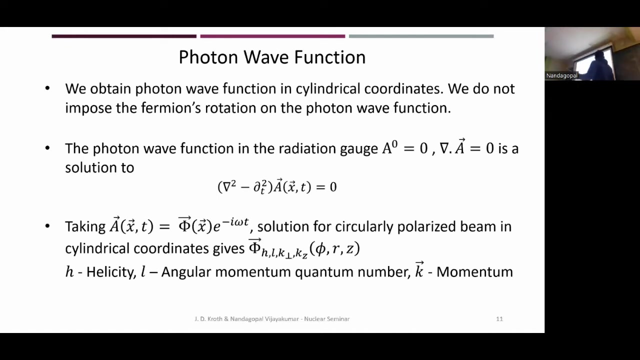 Now we'll be studying a spontaneous emission of photons, When, For me, on travels from when sperm and transitions from one level to another. so that means that energy of the initial formula will be greater than the energy of the final. Now the second step is to obtain the photon wave function, which is pretty standard. we use the radiation gauge and solve the Maxwell's equation, but the one thing is we'll be solving for the vector potential in cylindrical coordinates. 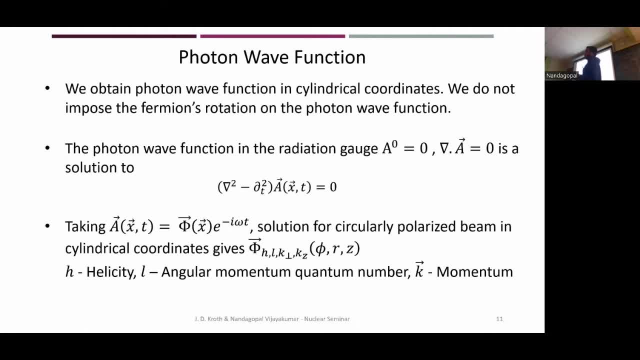 And we will not impose the fermions rotation on the photo. so we'll be obtaining the foreign wave function just in cylinder before. And so the wave function. Where we look at the wave function, it has for certain circularly polarized beam and has the following: one number, sketching health city and the angular momentum and create the momentum. 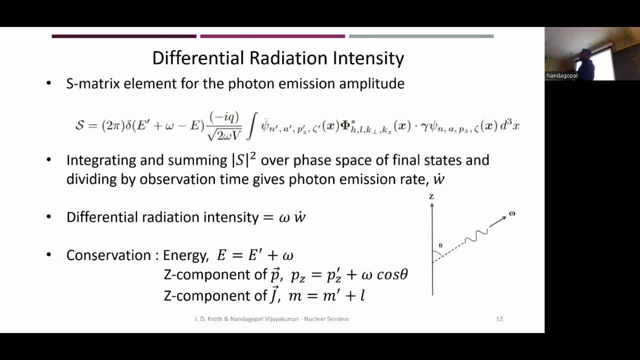 So once we have all the way function, The next step is to calculate the S matrix, and So we have a way function of the initial formula. you know, without the primes they function. final formula with the primes and the way function of the portal, and with that we get rid of them as an element. 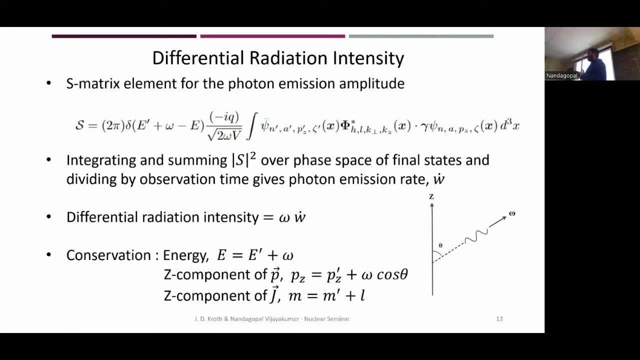 And which gives us the amplitude of photon emission from one specific level to another. So Once you have The S, Integrating and summing all of more square, or all the final state quantum numbers will give us the probability of Radiation. and dividing by total observation time uses the photon emission rate. 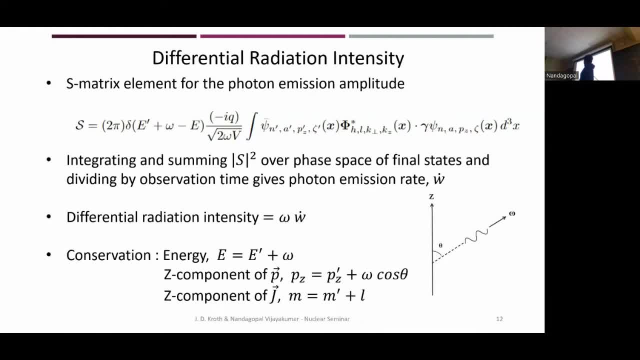 Multiplying this, But first of all explicitly shown in the X matrix element, is the conservation of energy. so the energy of the initial Fermion equals the final final plus that of the photon. The C component of momentum and total angular momentum are also conserved, as given by these equations. here theta is the angle of emission of the photon. it's the angle the photon makes with the Z axis or the axis of rotation. 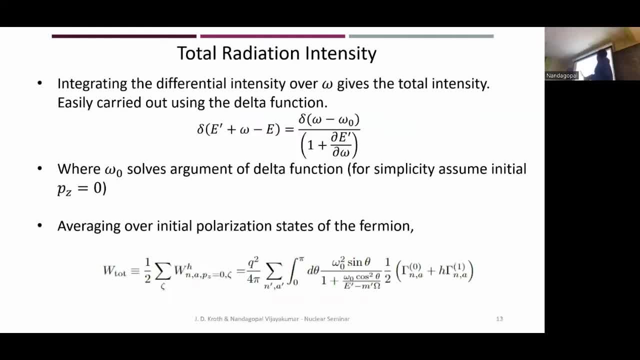 Now, once we have the differential radiation and three get top radiation density, we need to integrate our all Omega. and that integral is trivial: you can simply make use of the delta function that was there and this metrics And once you must add that a little bit and work with this simplified form in terms of Omega, where Omega notch is. 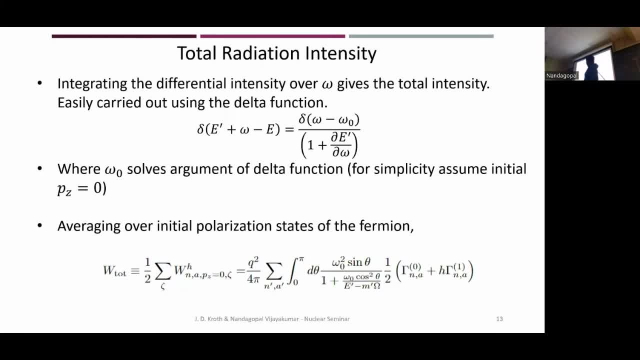 The value of Omega. that solves for the argument being zero on the left hand side of the equation and And for: in our calculation we assume that the initial C component of the momentum for me on the zero. because we obviously have translational symmetry along the Z axis, you can always choose boost into a frame such that the initial formula does not have a C component of momentum. 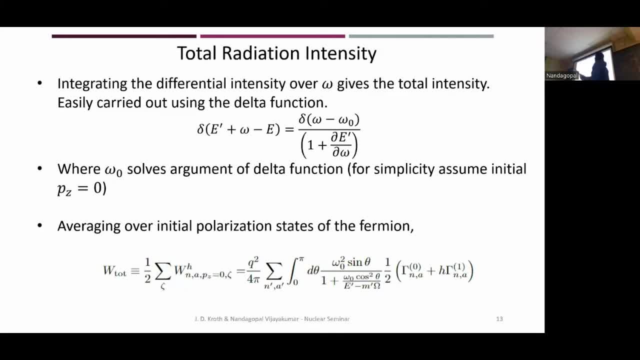 And so once he put plug in all the bay function and calculate, we will end up with the total radiation intensity of for a given initial stage. for me, on under rotation, producing the radiation- We also have Z terms- is the polarization of the fermion. 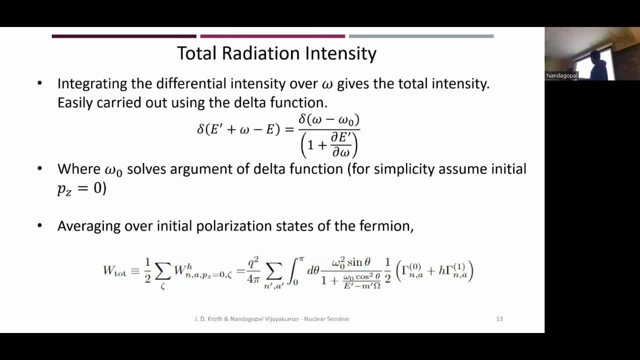 We need to. So we'll average all the initial polarization states to obtain the total radiation density, And that is shown by this expression, and here the gamma, gamma terms are what we obtain at the end of what we had in the previous slide. 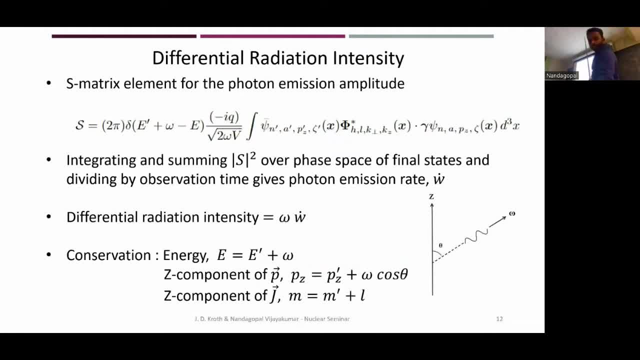 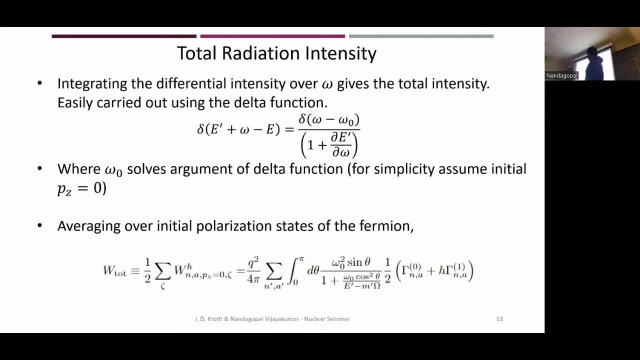 or everything in this integral. this boils down to what we have here, that is, gamma, and we can see here that we still have some over the final state phone numbers and primary prime and an integral over The emission angle. This is as far as we can go analytically. 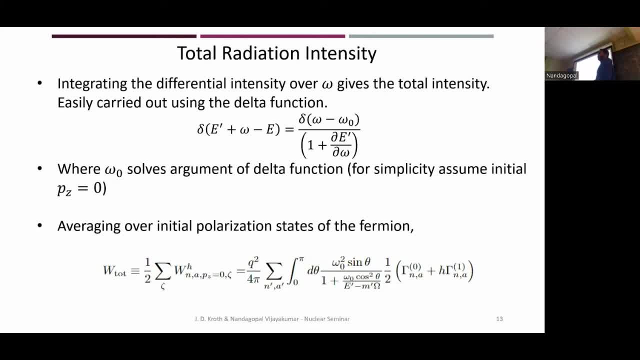 Remaining move forward, we need to use numerical techniques, which JD will explain shortly. This, so this brings us to the end of the first part of the talk. are there any questions? yeah, You The For this, this gamma. this is a shorthand notation for the final expression that we obtained. 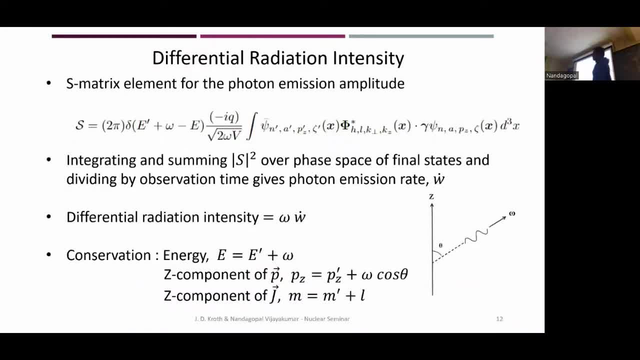 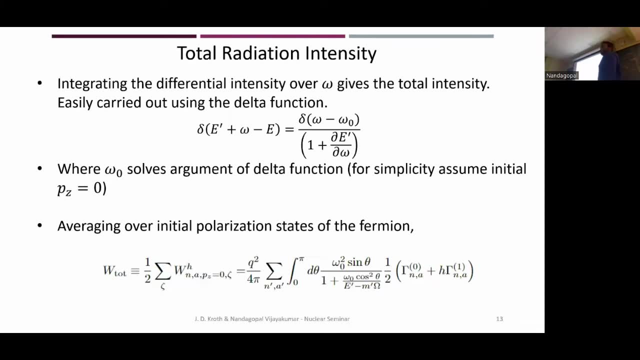 So we started with this expression for the S matrix and When we Log in all the way function elements and Some over The, the initial polarization, we get these two terms, These two curves: forms the initial fermion polarization. No, no, it's not the gamma function. 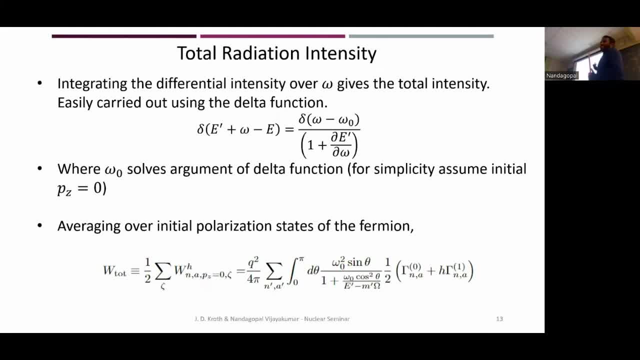 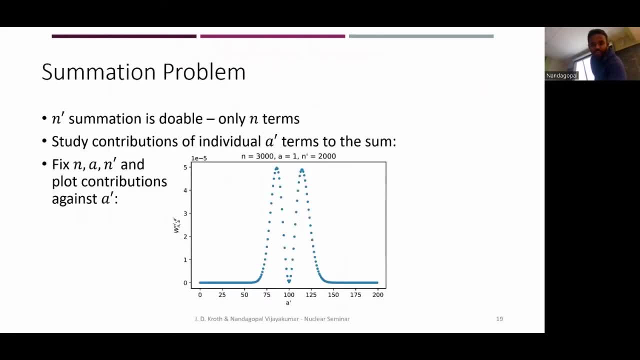 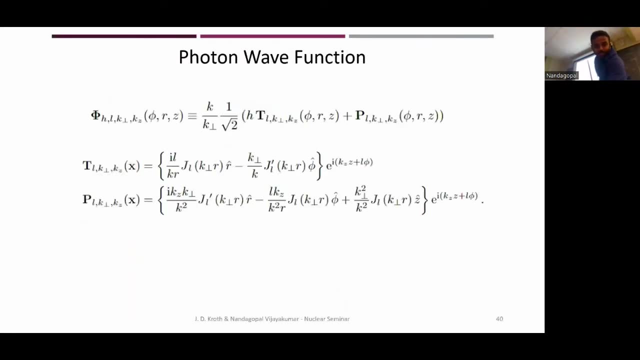 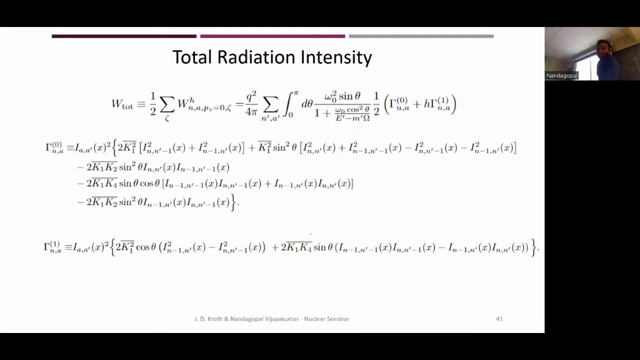 It's a complicated function that just shortened. If you wanna skip to the end, Yeah, I can show you the expression: Spoilers, Spoilers, Yes, spoiler alert. Yeah, these are the Yeah, Yeah, Where the constants are also new. 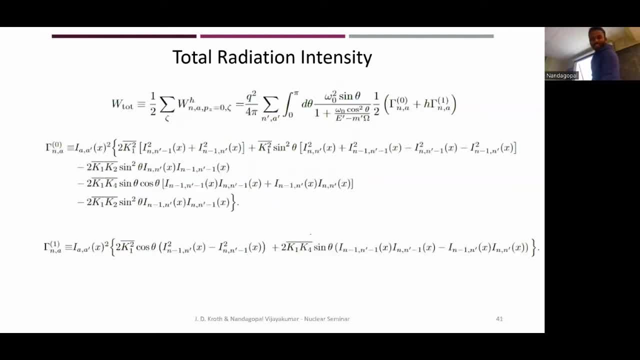 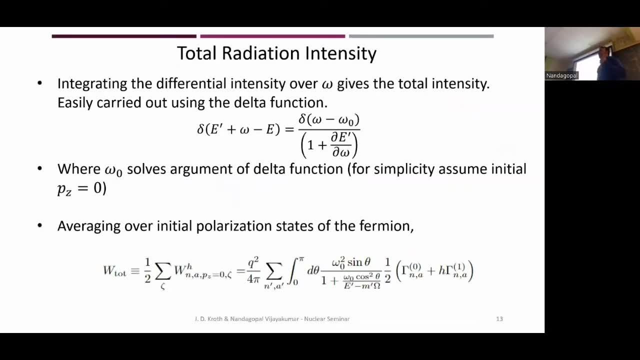 Anyway, it's just a simplified expression, But then, Yeah, Any other question? Okay, Then I'm gonna give it to JB to come to the talk. Okay, Thanks for the introduction. That archive link seems to not exist. 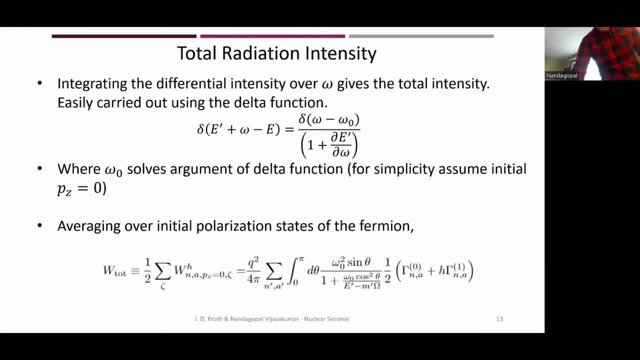 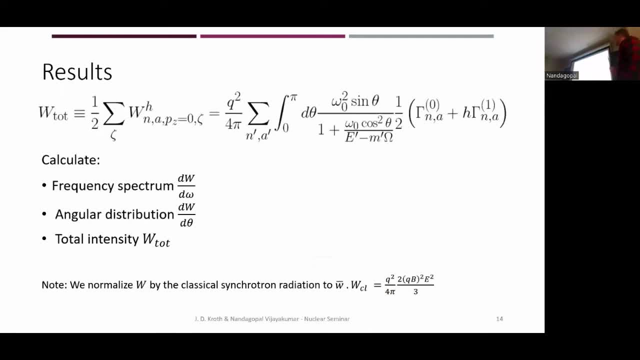 No idea where that number came from. I will investigate later. So my half of the presentation today will be about talking about the results that we get out of this analytical form, taking it, converting it into some numerical things, And so the things that we were interested in over the summer. 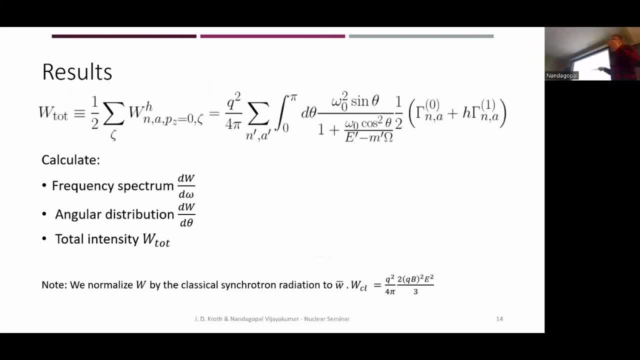 we're? what is the frequency spectrum? What energy do these photons have? what is the angular distribution? Where are these photons going and what's the total intensity once we integrate over omega, add up all the final states and integrate over theta? how much energy is being put out of here for unit time? 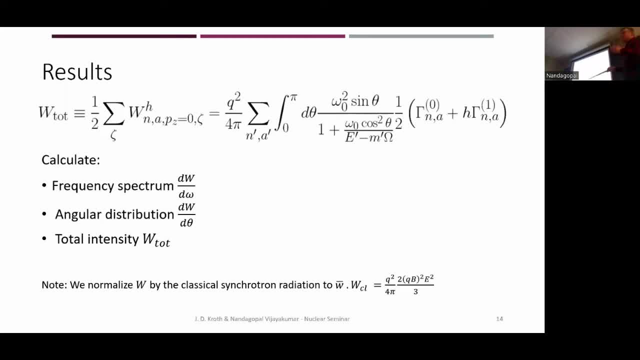 And they another notes we do. we'll be reporting our results as normalized, to the classical intensity, Yeah, which is important to note that it is proportional to the energy of the photon or the fermion squared, And so there's some. The radiation will seem to decrease at higher energy. 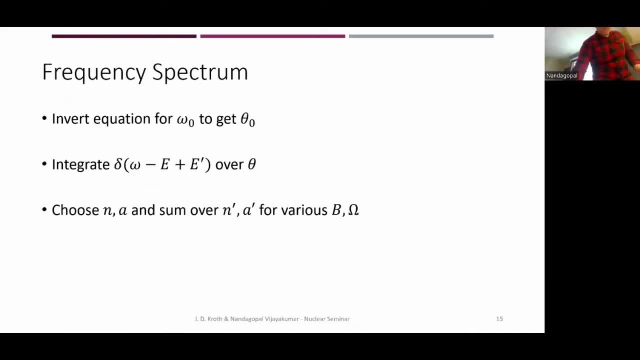 That's just the suppression in that normalization, And so first I'll discuss the frequency spectrum, And so to do this, we're going to actually go back a few slides to the S matrix And, instead of integrating over omega to get the funk, to get to enforce that the radiated photon has this omega, not frequency. 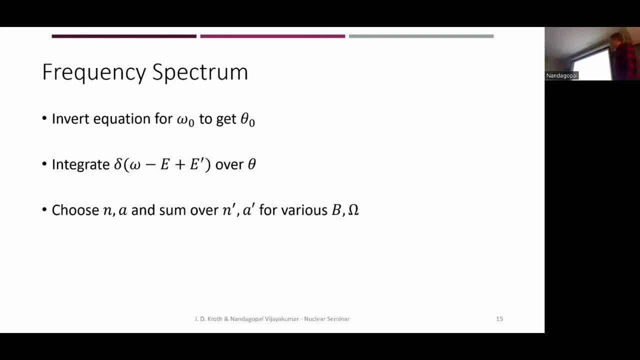 we're going to instead integrates over theta and enforce that it is emitted with a certain theta not. So, given a initial set of quantum numbers and a final set of quantum numbers and a frequency that we want, what is the angle that that will be emitted at? And so then we integrated over the delta theta. 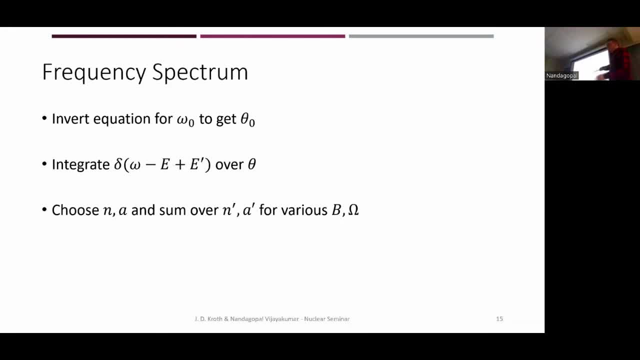 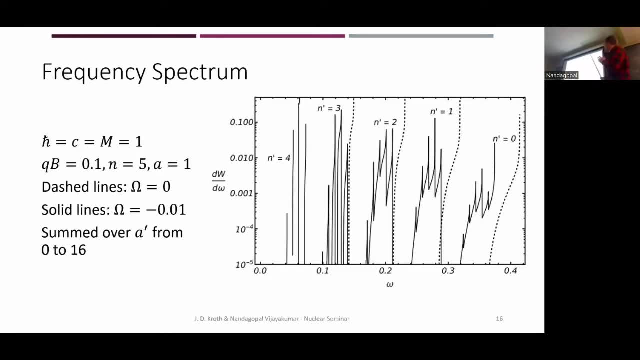 But using the delta function, and then we see what happens when we choose different parameters, And so, doing all that, we get this plot, And so this is a kind of characteristic frequency spectrum, The first. the dashed lines here are the case, without any rotation. 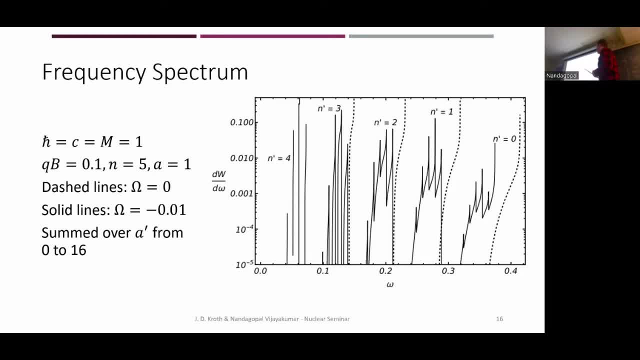 There isn't one over here- to this- and prime equals four island, because it's just about the page. Each final state and prime corresponds essentially to an island of peaks in the spectrum, And what it turns out is that each of these peaks correspond to a specific final, A prime value. 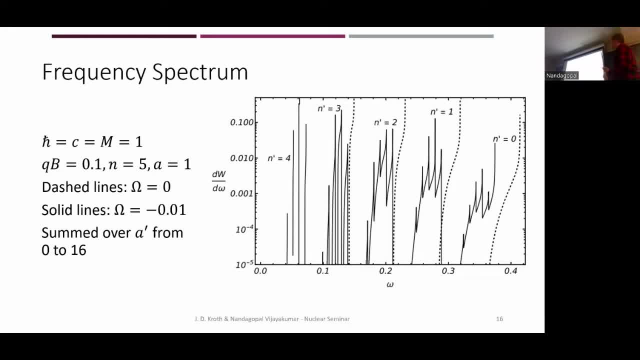 So because we have lifted the degeneracy in M, represented by having only one line for each N prime, we now have no degeneracy in M or A, And so we have a dependence of the emitted photons on that number. It's also important to note that you can kind of eyeball it here. 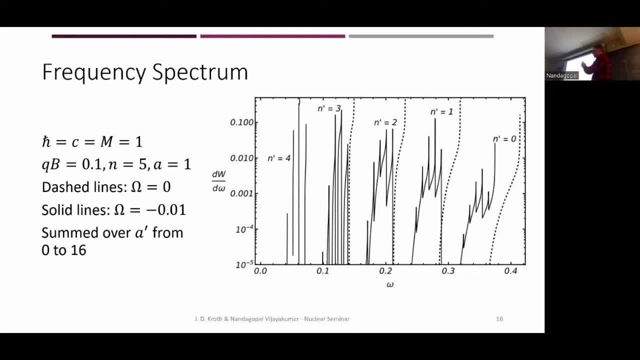 but these maxima of the peaks are roughly equally spaced. Each spacing is about omega, Each peak is about, shifted down by M omega from each non-rotating case. And finally, we only sum over a few of the allowed A primes here. 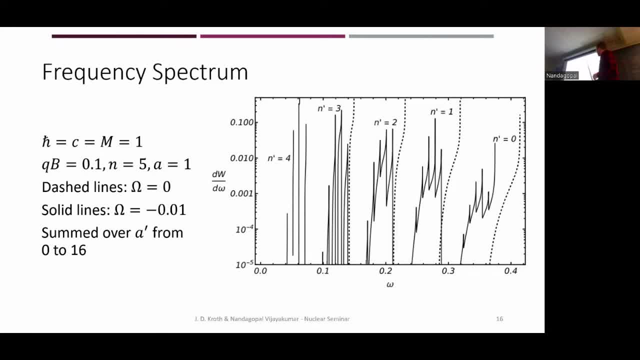 A prime can be any integer as long as our energy is equal to zero. Our final energy is less than our initial energy, And so we only sum over a few here. but it's OK, because we can see that as this goes down, this corresponds to increasing A. going to the left, we have decreasing amplitudes for each peak. 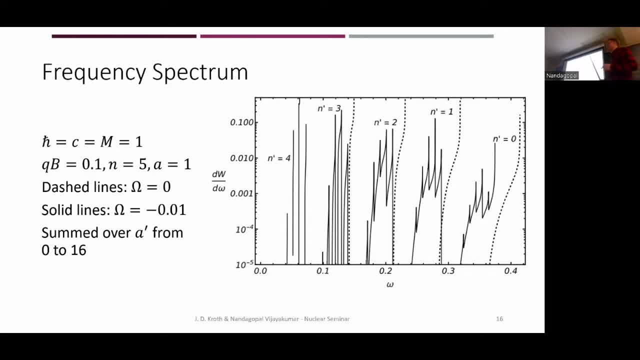 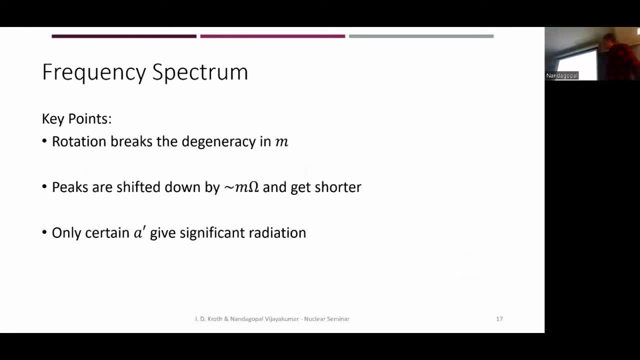 And so there is some dependence on the amplitude of the actual emission on A prime. And so, just to reiterate the key points, we break our degeneracy in M. That's something that we can see in the spectrum. Our peaks are shifted down by roughly M omega and they also get shorter. 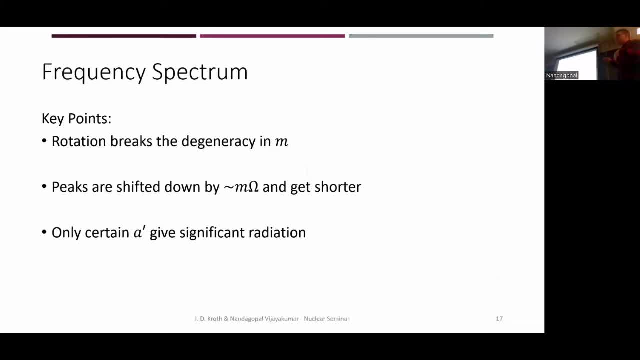 There was one line that was taller than the rest. That was the no rotation line, And essentially we're splitting that up into many peaks in the case with rotation. And finally, only certain A prime give significant radiation. And that last point is a important point to make. 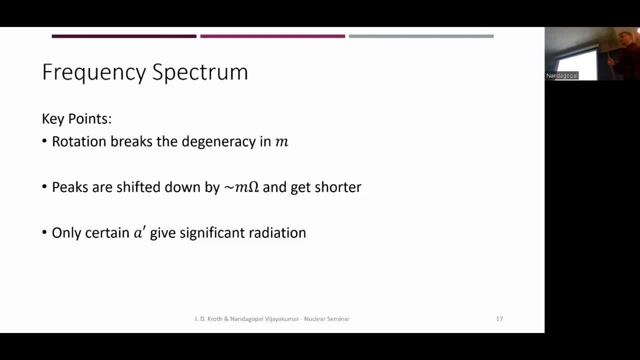 because in that summation over N prime and A prime for our total radiation, N prime has to go up to roughly N. A typical value for the initial quantum number N is a few thousand, But we also need to sum over A prime. Now, in the case of no rotation that goes up to infinity. 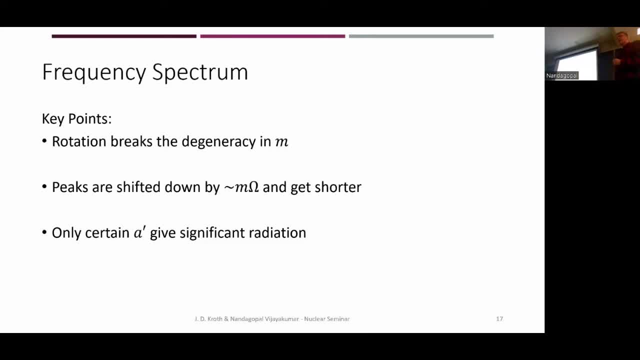 And we can do it analytically, because there's no dependence on the emitted photon frequency, on that quantum number, But here with rotation there is, And so because of the causality and boundary conditions we have to cut that off at A prime roughly a few hundred thousand. 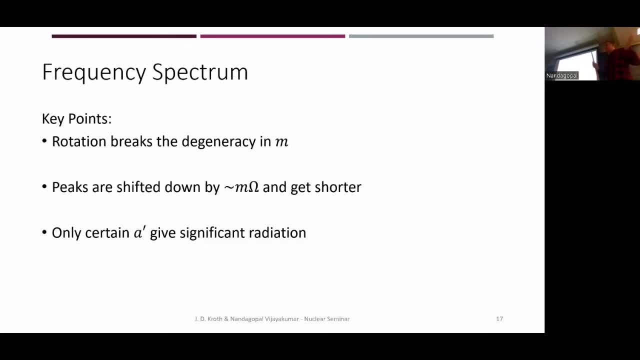 So we have roughly a few thousand N prime peaks or N prime final values times a few hundred thousand final A prime values. Multiply those together and it's a few billion terms in that sum that we had in the previous page And that presents a significant numerical problem. 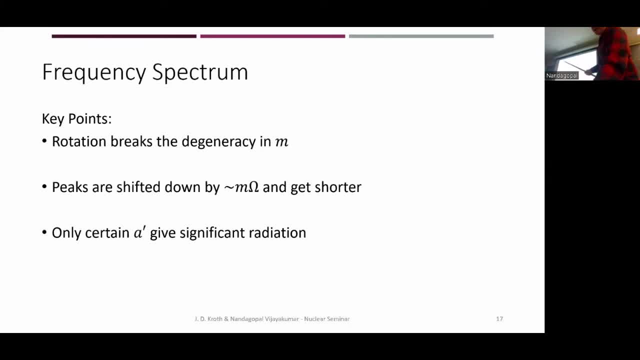 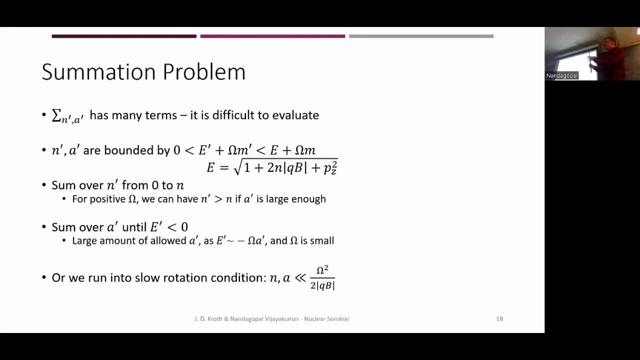 Because it's hard to do any of that analytically, And so this is the point I was just trying to make. There are a few billion terms in that sum, And each one of those is an integral, But the integral is the least of our problems. 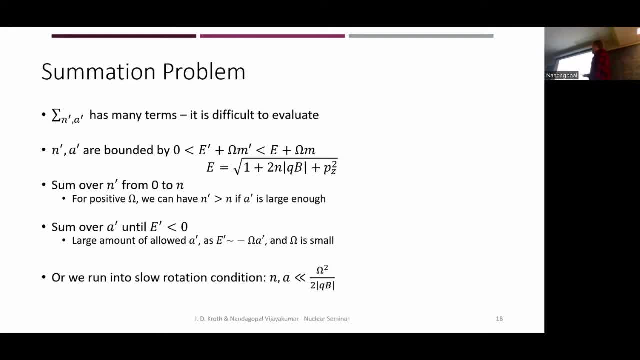 So N prime and A prime are essentially bounded by saying: our final photon or our final fermion energy is less than our initial fermion energy And it's also greater than zero. When we sum over N prime, we just go from zero to N. 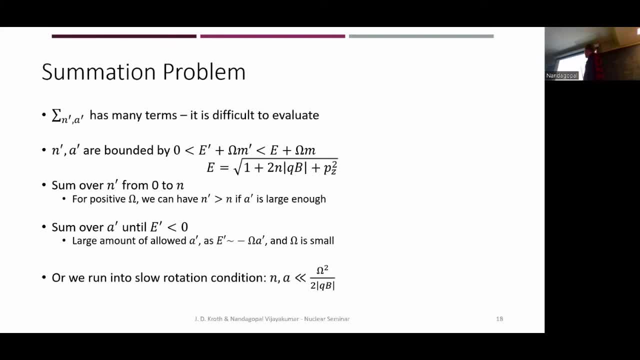 That's pretty straightforward, That's a few thousand terms, That's nothing. However, if we crank up A prime, and that's down here is energy is roughly or goes with minus omega A prime, We can push down the energy enough if we make A prime large to make N prime greater than N. 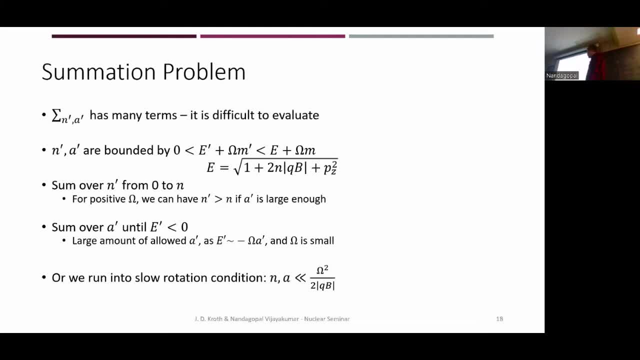 which introduces another whole zoo of terms to add. Investigating this, it seems like the A prime required is very large, which runs up against our essentially boundary condition that we talked about earlier, And also it makes the contributions to the sum very small. 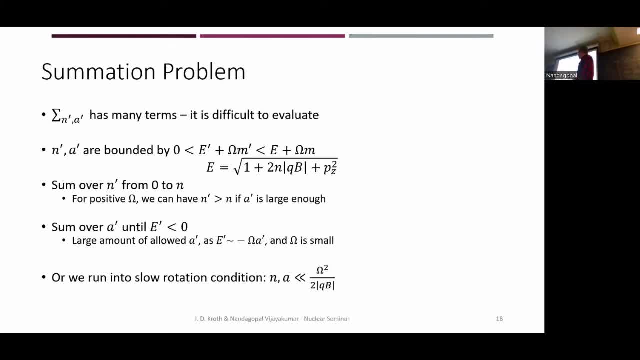 So cross that one out. Now all we need to do is sum over A prime until E prime is less than zero, Because omega is small and the energy has a term of minus omega A prime. that's going to happen very slowly And again we get a few hundred thousand A primes that we have to sum over. 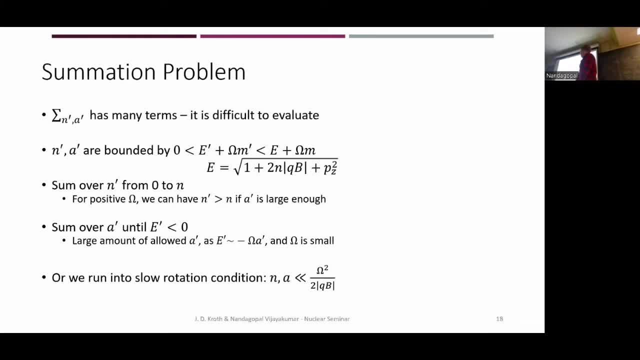 And we could do all this or we'll run into our boundary condition, where this is a consequence of our boundary condition that our N and A or N prime and A prime have to be much less than this ratio of lengths. And so, to tackle this problem, I looked and investigated. 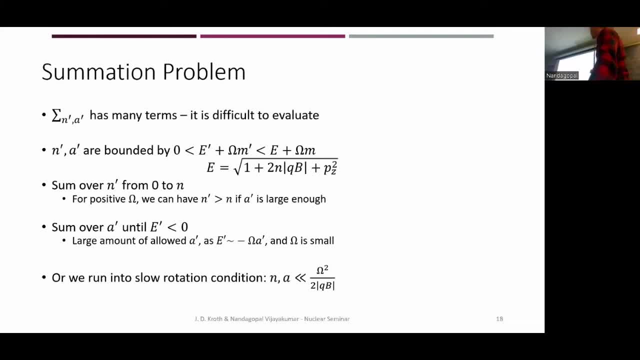 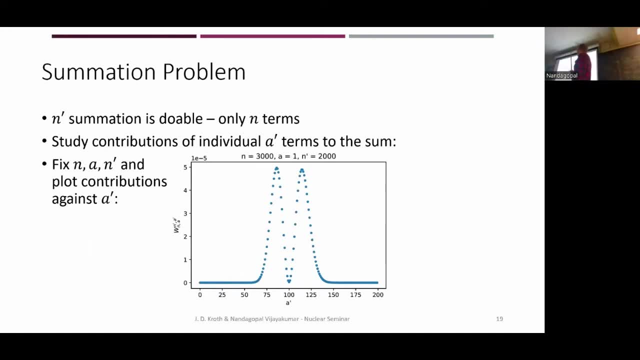 what do these contributions actually look like? So if we fix essentially N, A and N prime and just take the integral for a bunch of different A primes and plot it, what does it look like? So here we've got about 200 values of A prime. 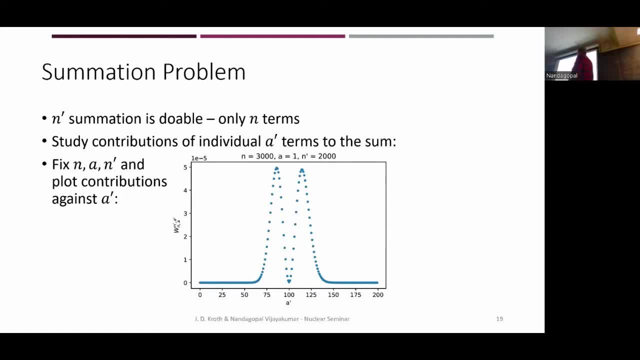 There are a few hundred thousand more that I'm not showing you and I didn't calculate, But it looks like there are only about a hundred or so terms that we actually want to calculate or that we might care to calculate, depending on what tolerance we set. 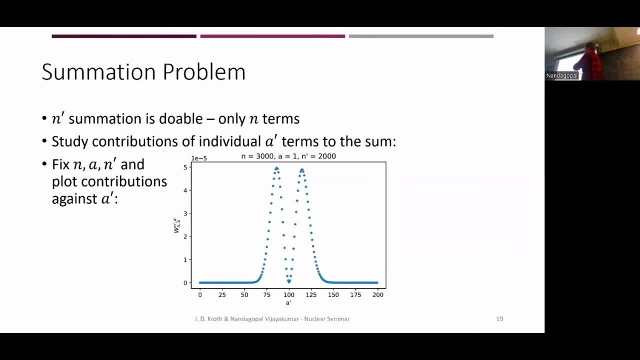 And so this is just a kind of characteristic one. Let's, if we could narrow a few hundred thousand A prime down to a hundred A prime for each value of N prime that we're looking at, that would be a great boon to our computational capacity. 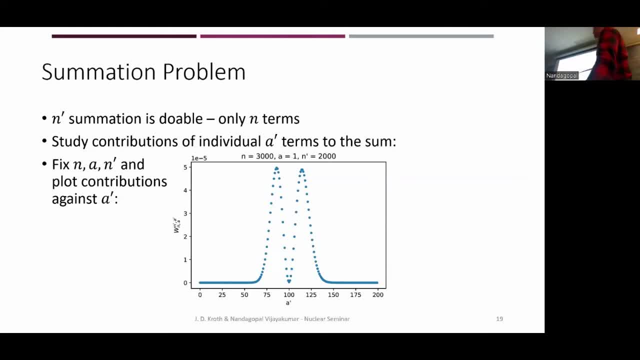 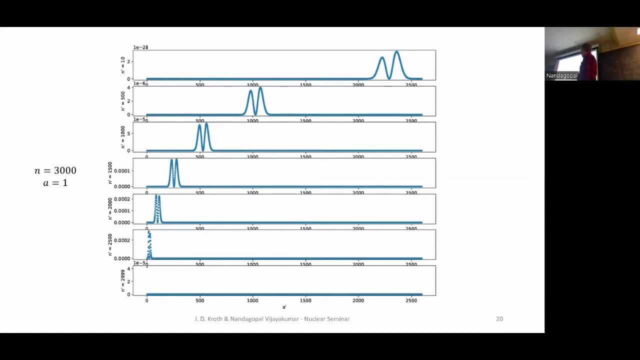 And so let's look at all this and now vary N prime as well and get a few of these plots, And so these are the same initial parameters. but now we've got multiple N primes. You're descending from the top or ascending N prime from the top. 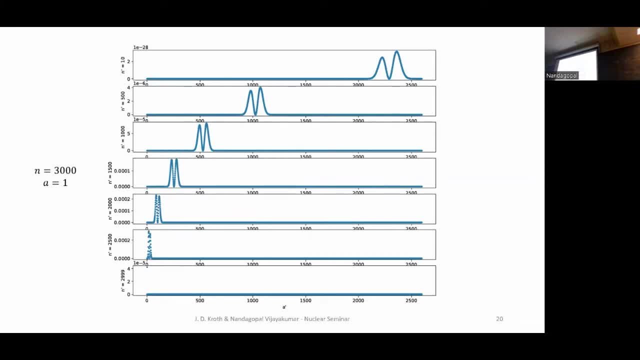 And so with N, prime is 2,999.. So one less than N, We have what looks like one significance, A prime contribution. Let's bring it up to 2,500.. We've got a few more, Okay, A few more, but kind of shifted over, for N is 2,000 and the trend continues. 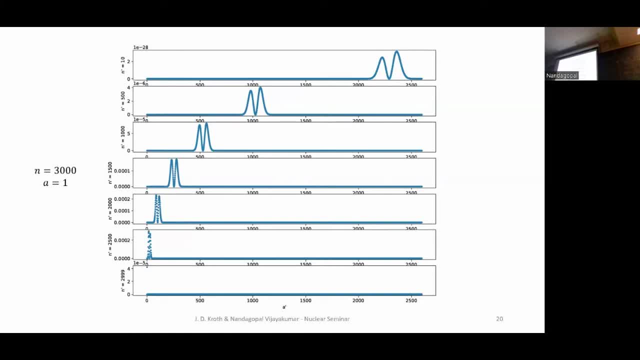 It's down this way. The omega dependence on there is somewhat interesting. It tends to make one of these peaks kind of more lopsided. The B dependence is essentially just changing the amplitude of each, Moves it around slightly, but the same characteristic features are all there. 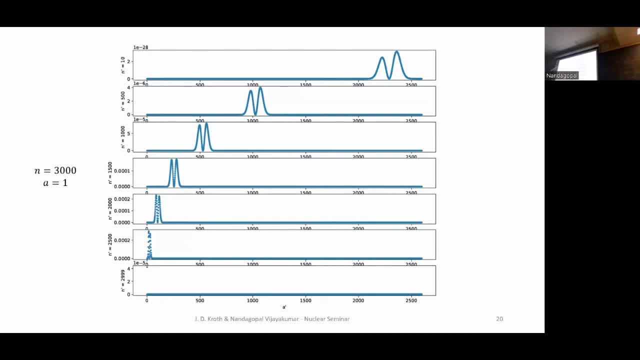 And so as N prime increases, we move things to the left, Towards. this is with A equals one, So it's kind of hard to see, or potentially hard to see. This is essentially just A prime is equal to A or thereabouts, And so we get again the comments that I just made. 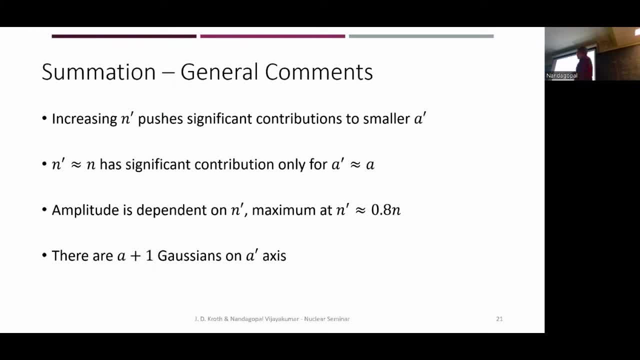 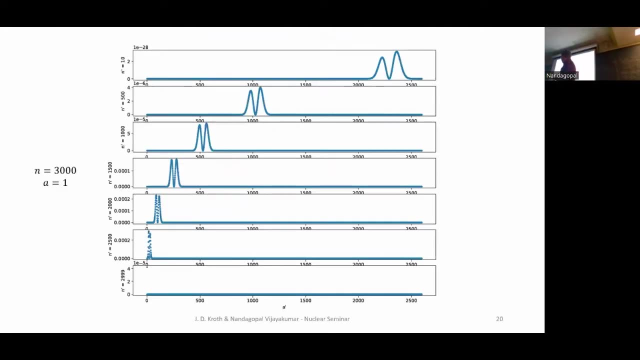 Increasing N prime pushes our sum contributions to the left. N prime equals approximately N Only has significant sum contributions for A, roughly A prime, And our amplitude is somewhat dependent on N prime. Go back here: Minus five, Minus four. 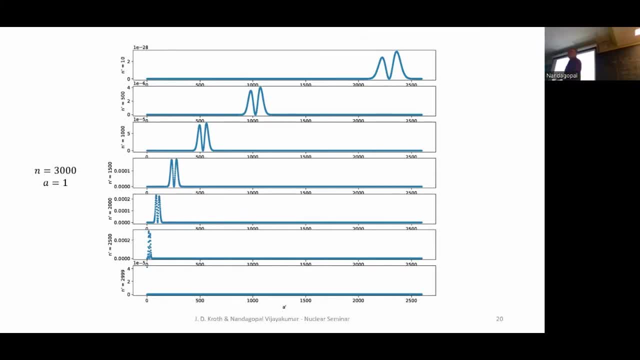 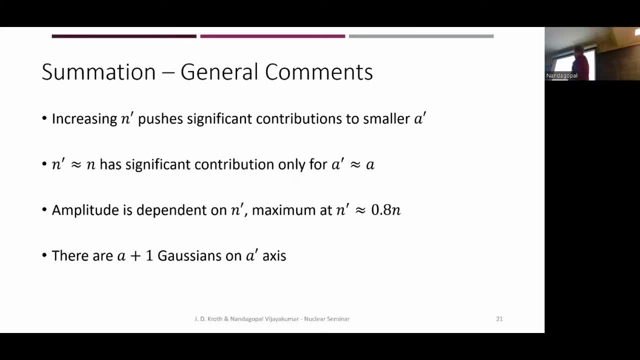 Minus five, Minus six And minus 28.. That's much smaller. If you look at the more data, you can see that it peaks at roughly N. prime is 80% of N. Not sure why. I did look for an analytical form to predict where these things are. 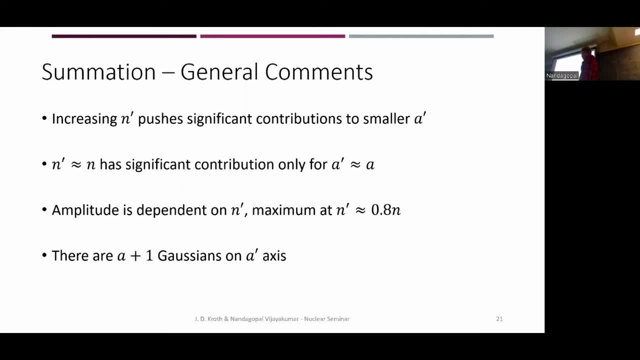 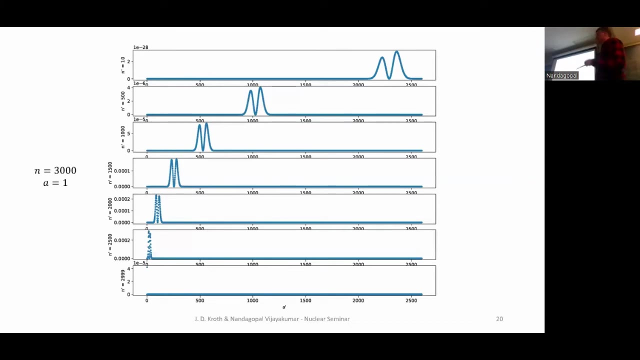 But nothing jumped out at me. But it turns out that most of your Ns- at least 90% of them- or most of your N prime values do contribute to the sum in a significant way. And another interesting fact that you get is that there are about A plus one of these Gaussian islands on your A prime axis for any given N prime. 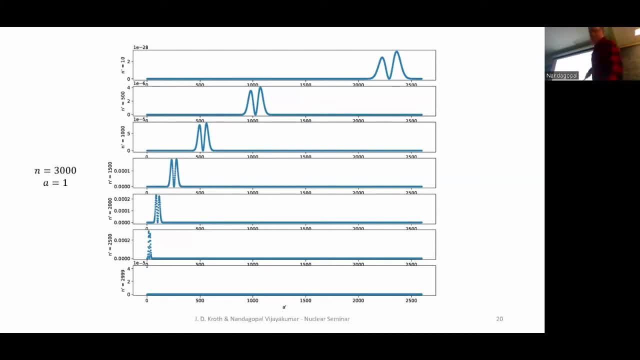 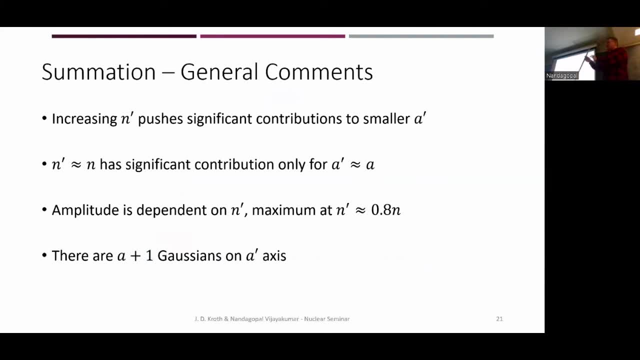 At least up to resolution, because these are discrete values And so with that knowledge we can kind of say, okay, there are only some places that we want to sum. We can't necessarily say, okay, where does it go up and then down however many times. 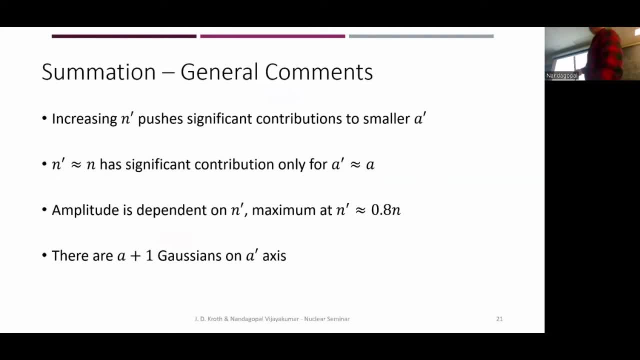 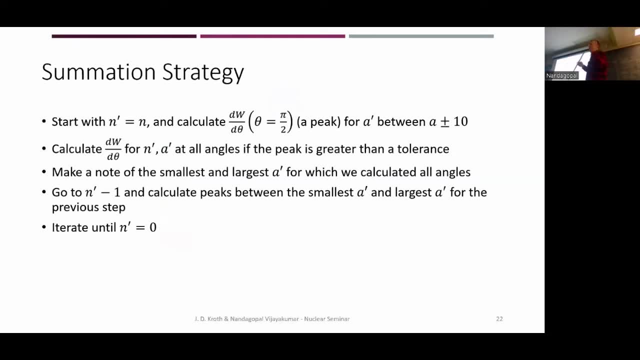 But this is the summation strategy I came up with. So we're going to start at N prime equals N, where we know where our significant contributions are. We're going to say: let's calculate at theta equals pi over two. In a few slides you'll see why I choose that, because it's essentially the maximum of the angular distribution for the sky. 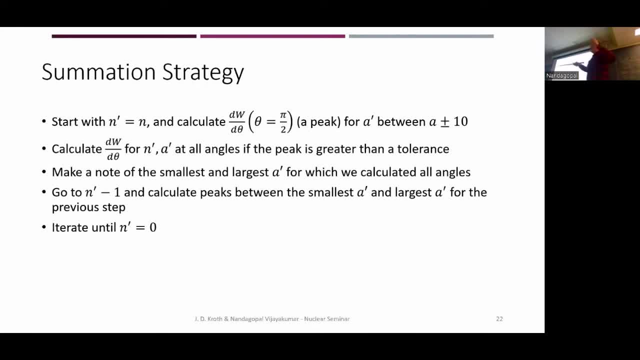 And we're going to do that for a bunch of A prime values. We're going to start with A and do plus or minus 10.. It can be any integer. We just want to give it some width so that we can capture any movement of these peaks. 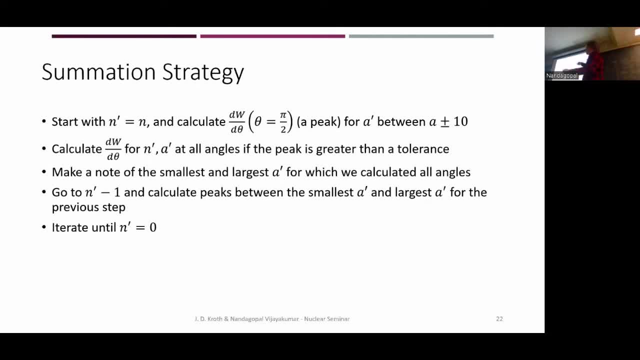 Now, if these peaks that we calculate are greater than some tolerance, Then we are going to do it. It all calculates the angular distribution for that term at all angles. Add it to our sum and keep going. Now we're going to make a note of what's the smallest A prime that we did that for. 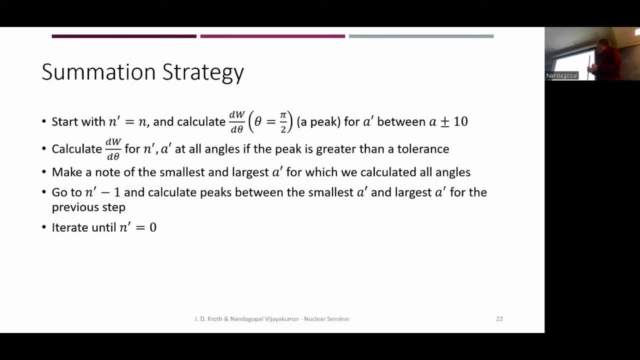 What's the largest A prime that we did that for And then make a note of that. Use that in our next step, where we go to N prime minus one, We're going to say, okay, we're going to start at the minimum A prime minus 10 or so. 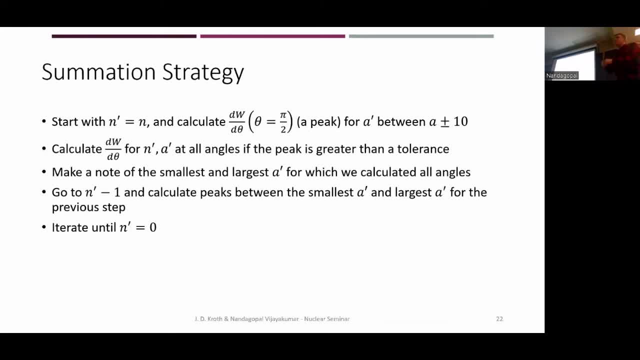 And then we're going to go to the maximum A prime plus 10 or so, Just to capture the width of the thing. And then we're going to keep doing that, Calculate peaks, calculate angles, and iterate until we reach the N prime equal to zero. 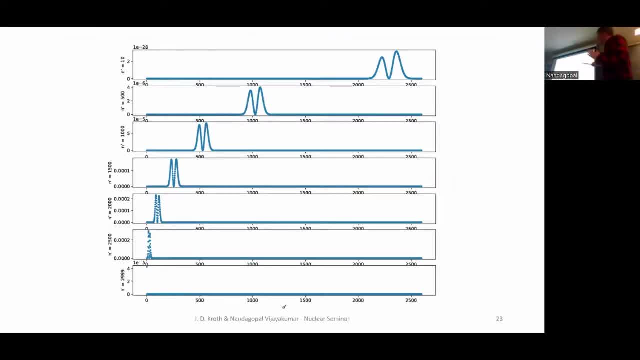 And so just a graphic of what that's doing. We're going to start down here at 2999 or 3000.. Draw a box And we're going to calculate the intensity at pi over 2 at that guy. We're going to say, okay, there's one guy there that meets our tolerance. 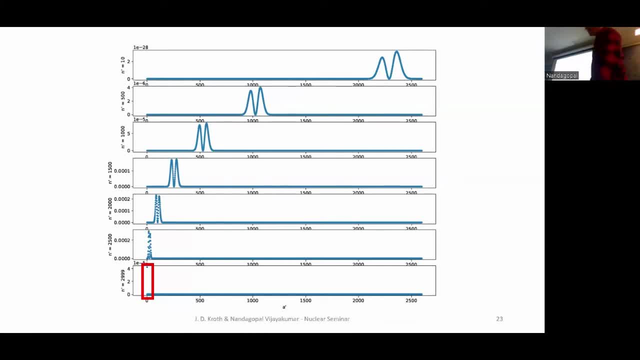 Let's calculate it for all angles And then note, okay, that's our minimum and maximum And go to the next step. Now we can move over a little bit because we know where that peak was And say, okay, let's calculate a bunch of peaks. 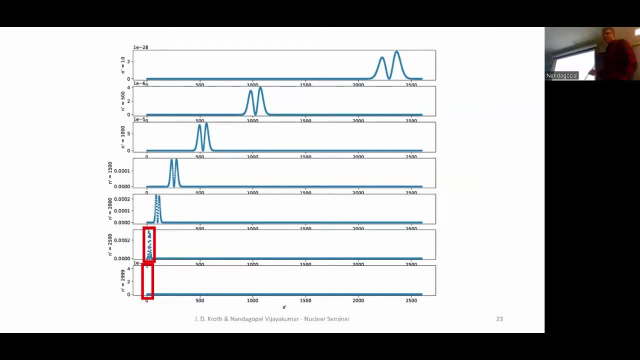 Let's calculate the significant contributions to the sum. Note where the minimum and maximum are. Move to the next step, And in doing this we can slide ourselves along the axis Without getting any of the unimportant or small- sorry, excuse me, any small- contributions. 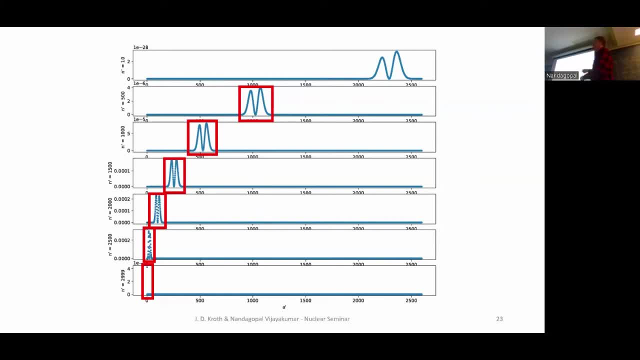 Because I plot out to A prime is 2500 here, But this axis goes all the way out to the cornfields- A few hundred thousand, like I said, And we get to move along our axis without any significant computational waste. And so, using this summation strategy, we can do the rest of our numerical analysis. 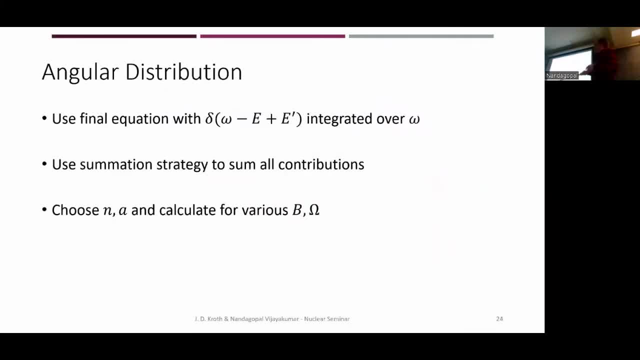 We're going to start by getting that angular distribution. We're just going to use our final equation that I had on my first slide and on the GoPro's last slide- Integrate over omega, And then we're going to use our summation strategy to get all the significant contributions greater than whatever tolerance we want. 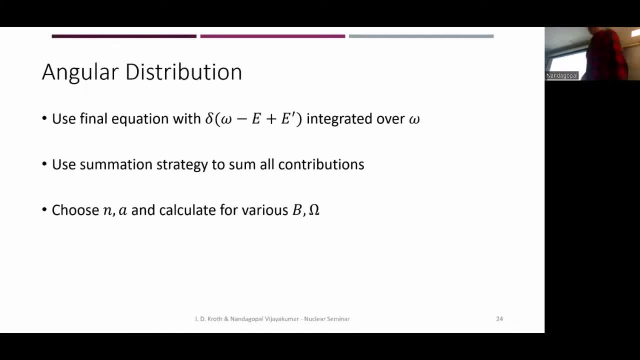 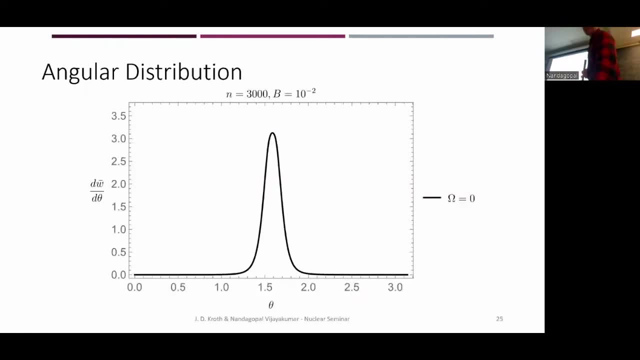 And then choose N and A, choose B and omega, see what happens. And so this is what we get, without rotation, Fairly unremarkable Lorentzian shape. I think this is the limit of what you get in, say, Jackson or something. 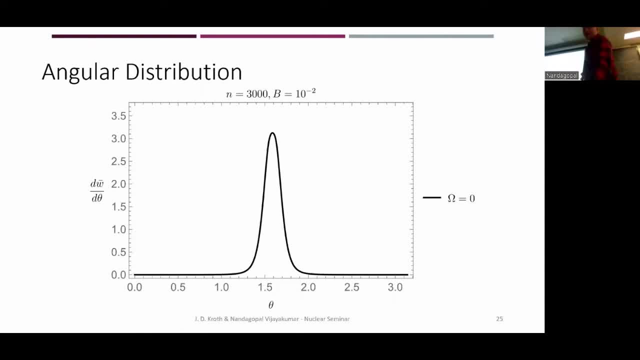 Now we're going to introduce rotation which is parallel to the axis. So omega and B are points, Omega and B are pointing in the same direction And we see an enhancement at all angles. basically Same characteristic shape but enhanced. And now if we have B going this way and omega going this way, we get a suppression by what looks like about the same amount proportionally. 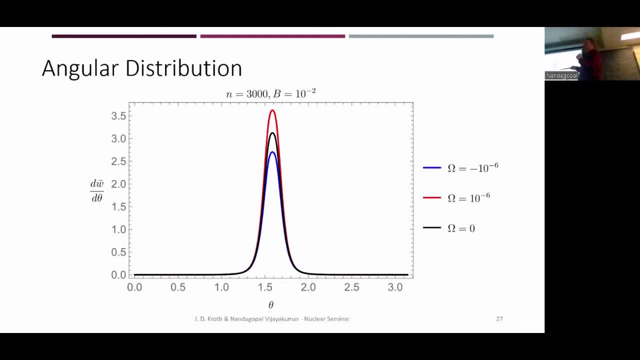 And so this is the big thing, Or the first glimpse of the big thing. Rotation with the field gives us an enhancement of the radiation. Rotation against the field gives us suppression of the radiation. We can do this for a smaller magnetic field, one order of magnitude less. 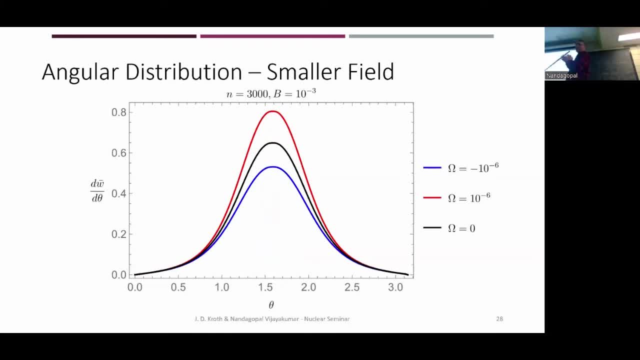 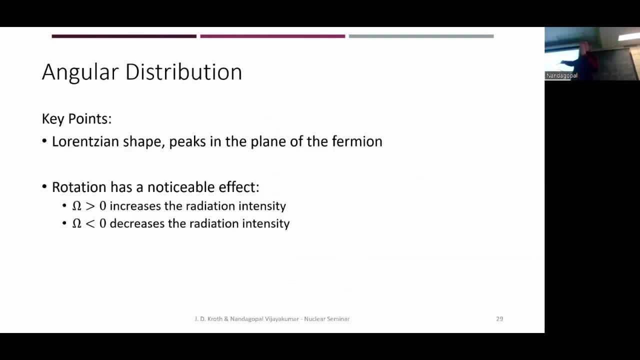 And we see the same thing just a little bit wider. It's lower energy And so the key points of that again Lorentzian shape, fairly unremarkable. But omega greater than zero with the field increases radiation. Omega less than zero against the field decreases it. 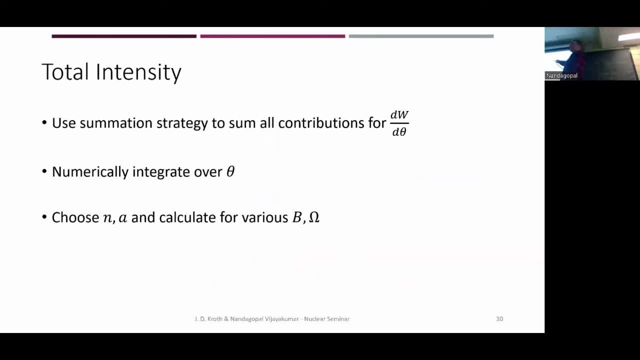 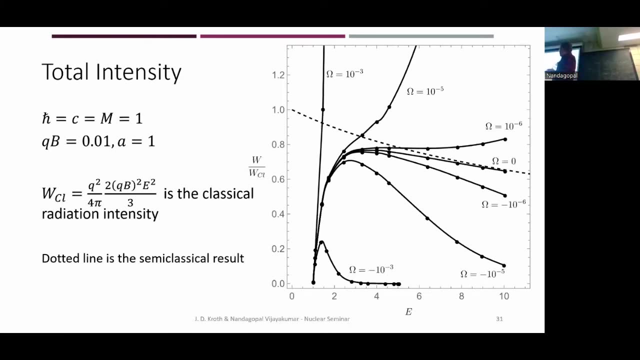 And so now we're just going to get into the total intensity. We're going to use that data that we got for the angular distribution, numerically integrate and see what happens for various input parameters, And this is the figure we get. So this is the total intensity normalized to classical intensity. 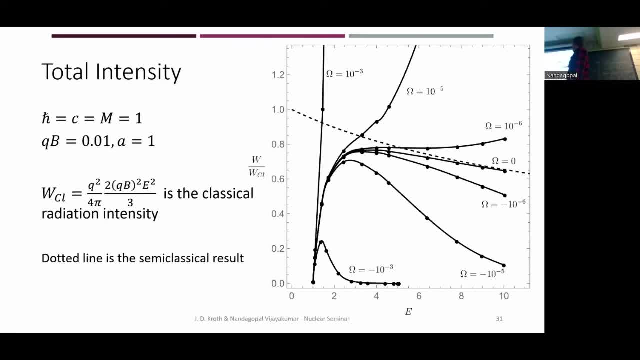 Here, or one of these lines. here is our no-rotation case. It approaches this dotted line which is our semi-classical results, essentially in high energy, where we say n prime goes to a continuum And we can integrate rather than sum. 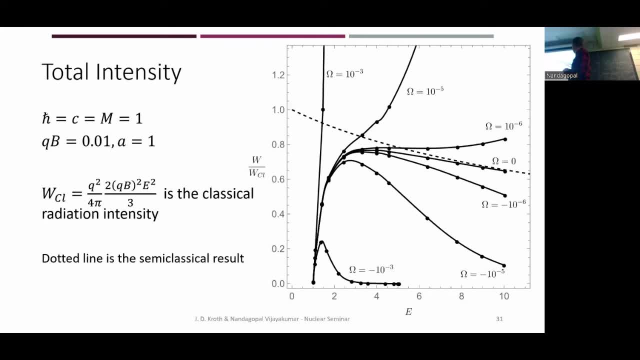 But the interesting things are these guys right. So with the same magnitude of rotation we see enhancement and suppression of roughly the same, And for slightly larger rotation- or slightly larger, but still fairly small, at least compared to QB- we get a pretty significant suppression at higher energies. 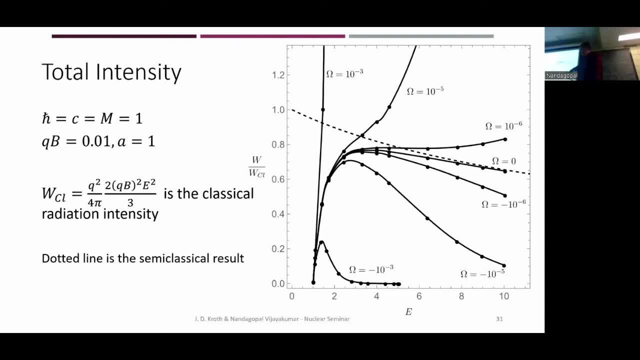 And with this rotation which is getting closer to saying our approximation is a little bit shaky. we get an almost total suppression even at lower energies. So that's what we get, Even at lower energies. The effect is also considerably larger for larger energies. 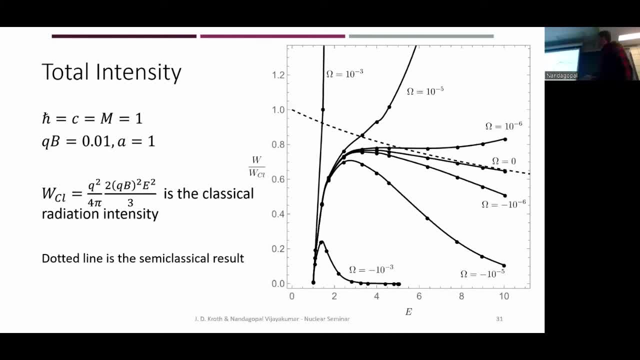 And these guys are mysteriously going off the page here. Sorry, JD. Yeah, So do you have these two lines for different percent? Oh, I didn't see the sign, Sorry, OK, Yeah, Yeah, The sign Yeah. 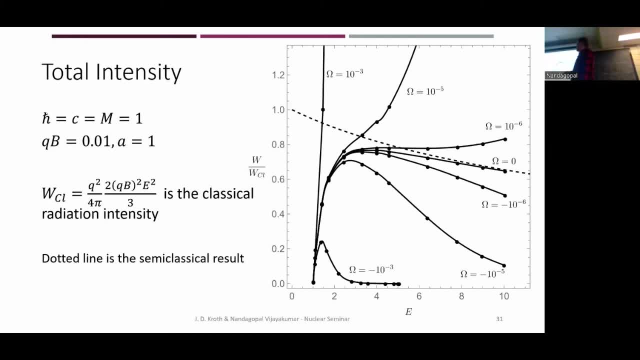 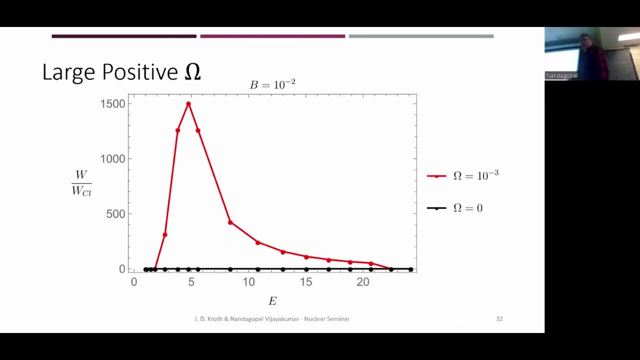 Note the sign here. Yeah, And so let's look at this guy. So the neural rotation case is down here. I will remind you of the scale 1, 1500.. Something big is going on here. It may be that our approximation is breaking down a bit. 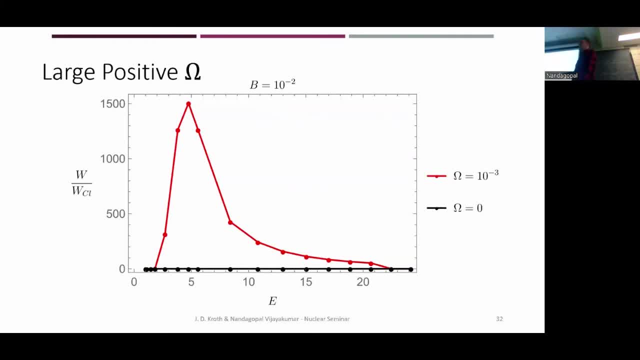 But the same behavior is seen of that 10 to minus 5 omega equals 10 to minus 5 line, Except that's a little bit shorter, but it's still increasing And our numerical results haven't returned a tail like this yet. 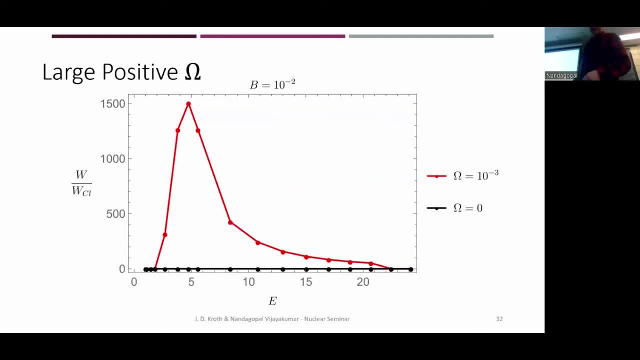 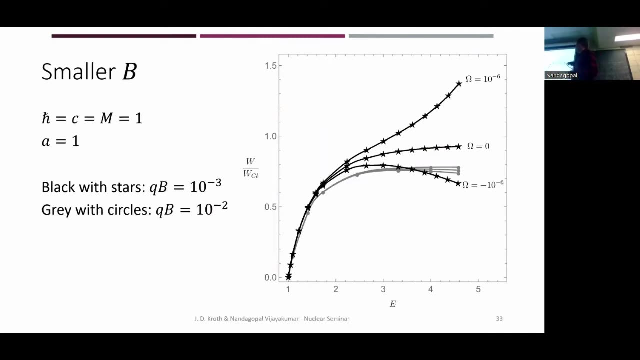 But there's no reason not to expect it. There's no reason to expect it. Let's go to slightly smaller magnetic field. So these black lines are the smaller magnetic field. These gray lines are the lines I showed you on the last slide, but at a lower energy. 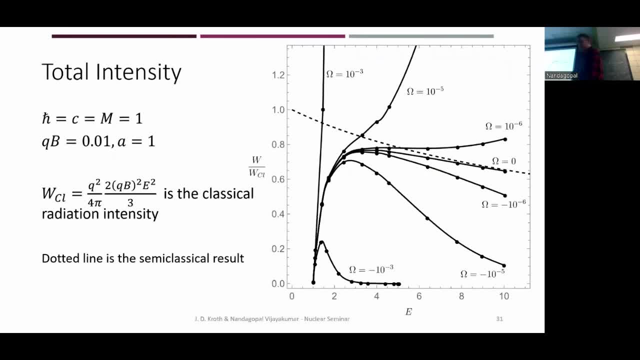 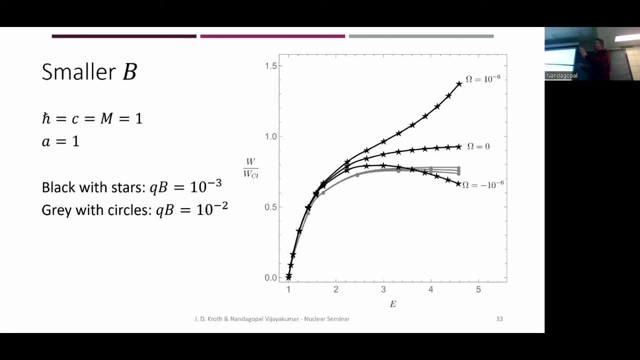 The last plot had energy up to 10. This one has it out to 5.. That's just because in that dispersion relation we had, E is roughly square root of 2N times B. The smaller magnetic field means we need to go to higher N, which means more sum contributions. 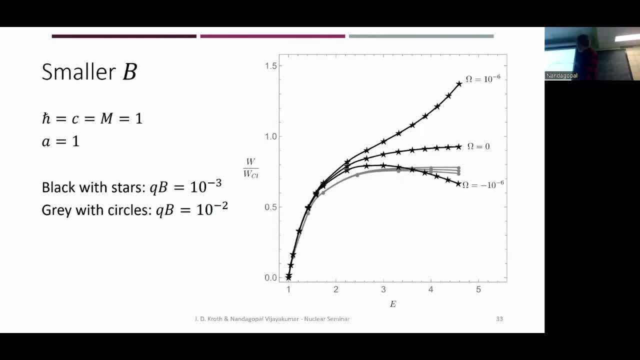 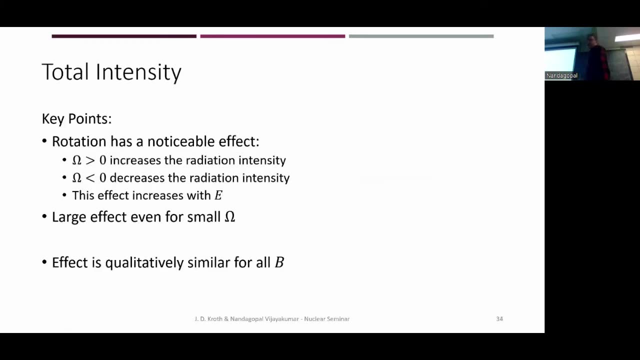 to compute, which means longer computation time. But at this lower energy we see the same characteristic behavior that we saw on the last slide Or on the last figure, for QB is 10 to minus 2 at higher energy over here, And so the main points to take away from that are that our rotation has a noticeable effect. 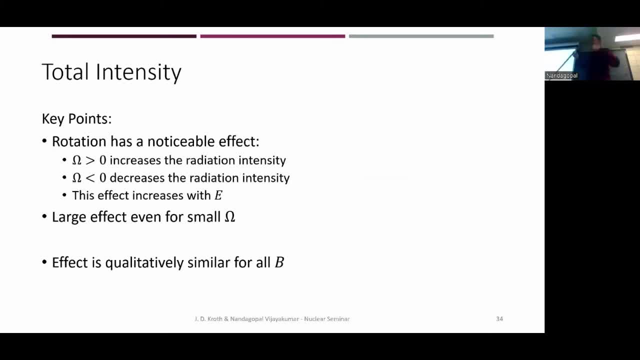 on the synchrotron radiation For omega greater than 0, we increase the radiation intensity. We saw that with the angular distribution and of course it carries over into the total. Omega less than 0 suppresses the energy, the radiation, and we see a marked increase for 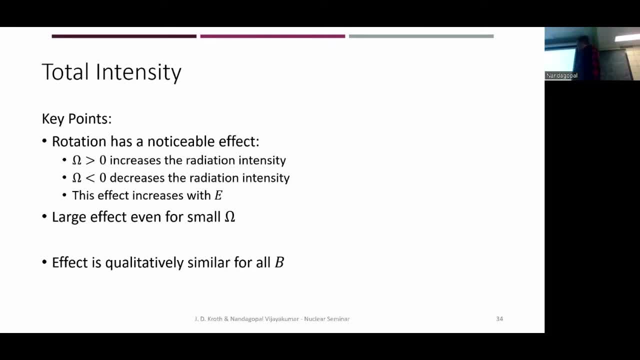 greater values of the energy, We also get a large effect for even small omega that we've been assuming we have, And we have qualitatively similar behavior of this effect for all magnetic fields, And so the last thing is we have a bit of a somewhat classical interpretation of this. 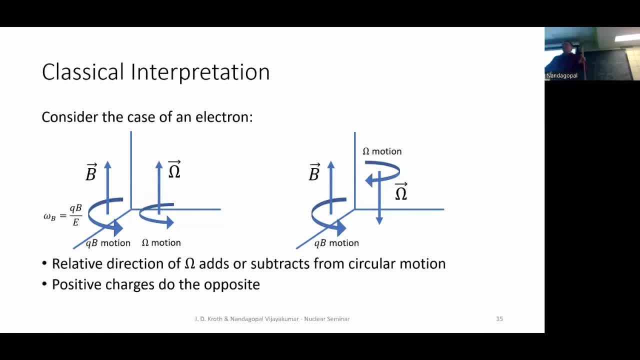 And so if we've got an electron and we place ourselves in this rotating frame, And when we let this electron go with the magnetic field, it's going to start going around in this direction. And so now we want to, or it's going to go around with the rotate, the synchrotron frequency. 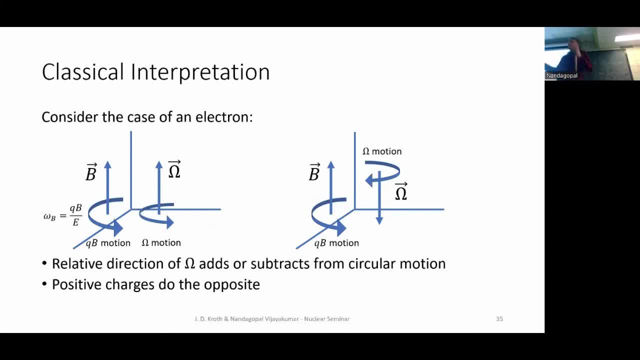 over there. And so now we want to get out of the rotating frame into our lab frame, And so while the electron is going this way and the frame is rotating in this direction, I'm going to rotate in the opposite direction to get out of it. 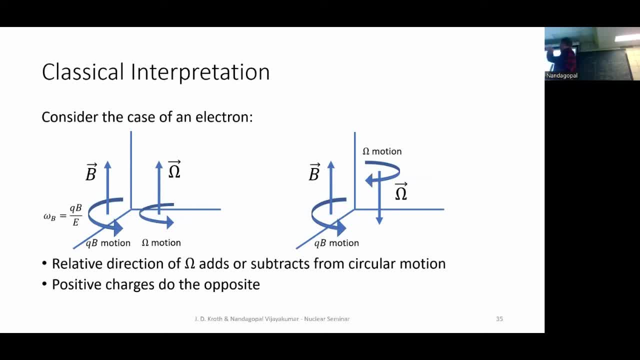 So my electron is going this way, I'm going to start turning this way And I see the electron must be going faster because I'm rotating essentially against the electron's rotation And so it's moving faster. It must be seeing a greater field. 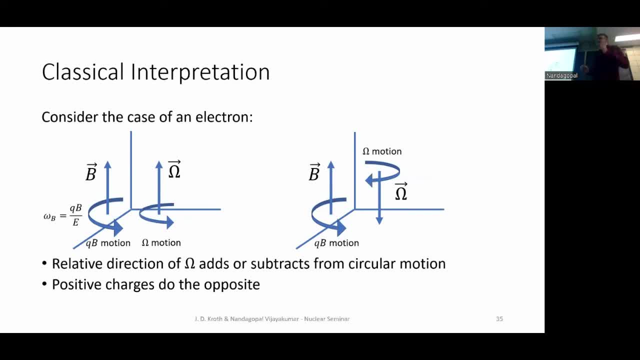 It must be radiating more, And that's what we see in the plot that I had a few slides ago. The opposite happens if the rotation is going the opposite direction. The electron is going this way. I'm going to rotate this way to get out of that field, that frame. 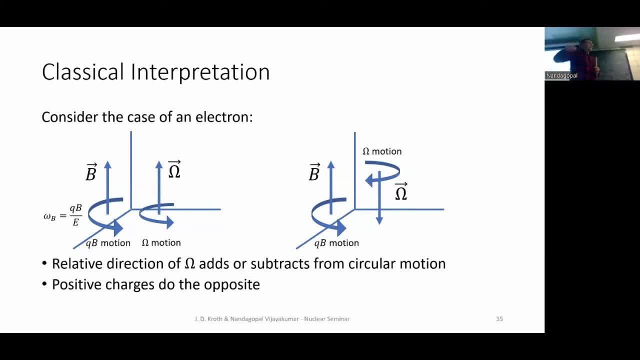 And the electron looks like it's going more slowly because I'm rotating this way while it's also doing that, And so I say the electron is moving more slowly, It must be seeing a smaller field, It must be radiating less, And so that's essentially what we have here. 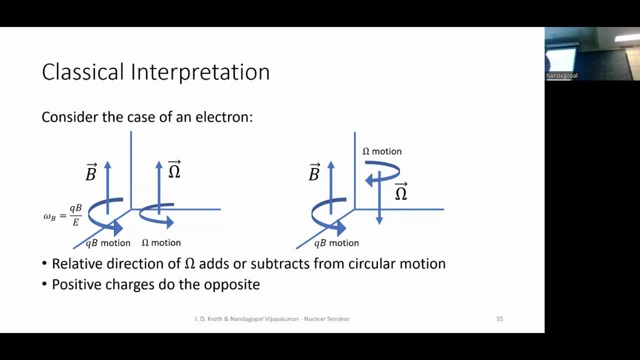 The QB motion, the synchrotron motion and the rotating frame motions add up to get a larger radiation. In the other case we have them essentially subtracted And the energy dependence of that, the falling off the greater effect at larger energy. 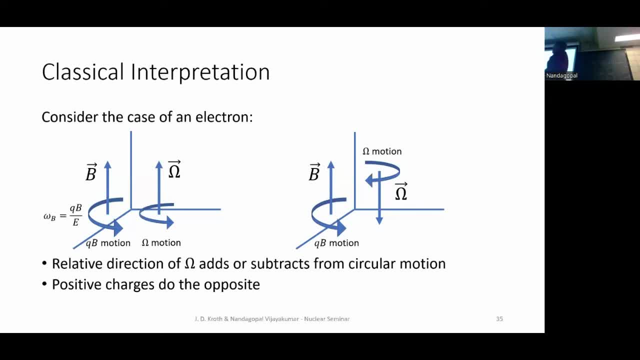 is essentially because this synchrotron radiation is equal to or proportional to one over the energy. So as the energy increases, this guy is going down while the omega is staying the same, And so omega B is getting smaller while omega is getting larger. 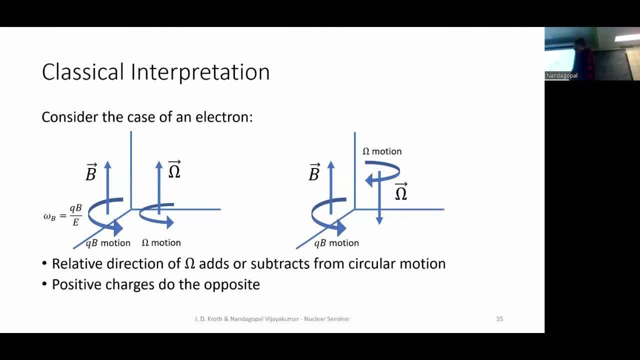 And so the effect is enhanced. Now, all that I said is essentially the opposite, for a positive and a negative. The positive charge because this guy is going to reverse. So if we all just turn our heads, we get this guy for positive charges, but this guy with 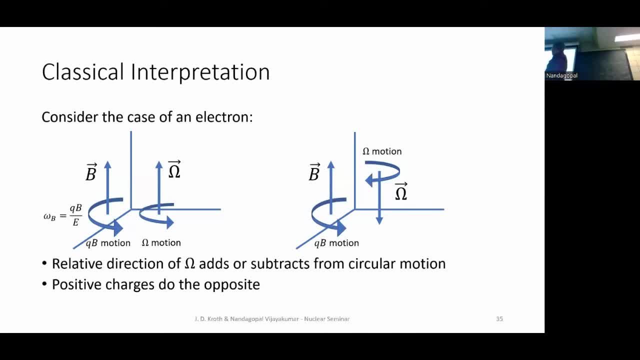 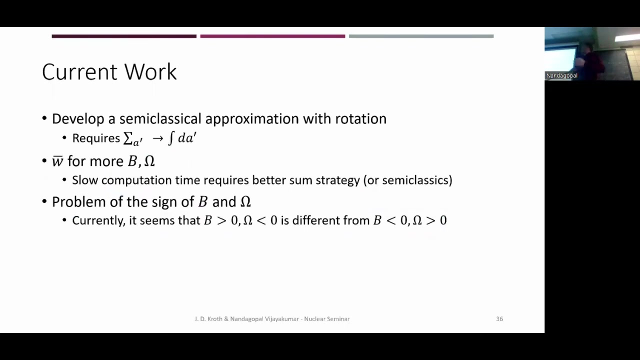 B and omega. aligned essentially for the positive charges, we get a suppression And with them, anti-aligned for positive charges, we get an enhancement, And so that essentially brings us into where we are right now. So our current work, Nandagopal's current project, is to say we want to do semi-classics. 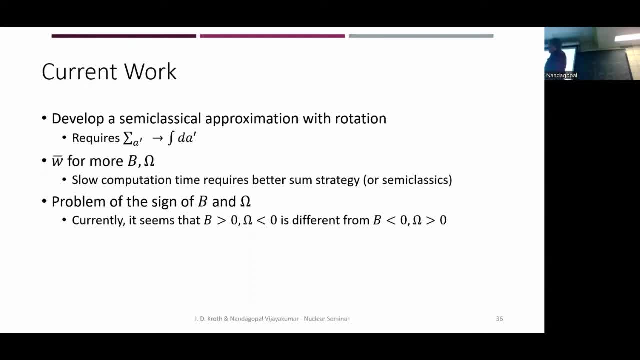 with this. We want to say in the norm rotation case we can do semi-classics and say the sum over n prime goes to an integral over n prime, which is much easier to do, And we want to do the same thing with a prime. 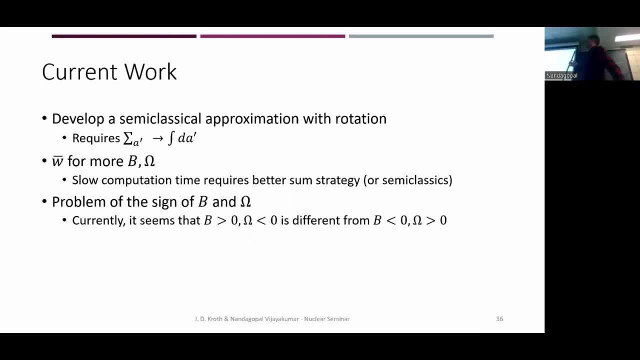 We want to say sum over a prime goes from the integral over a prime, And then that would significantly cut down on our computation time. Then we want to essentially make more figures, like the one that I showed of the total radiation, get more B and omega combinations. see what happens. 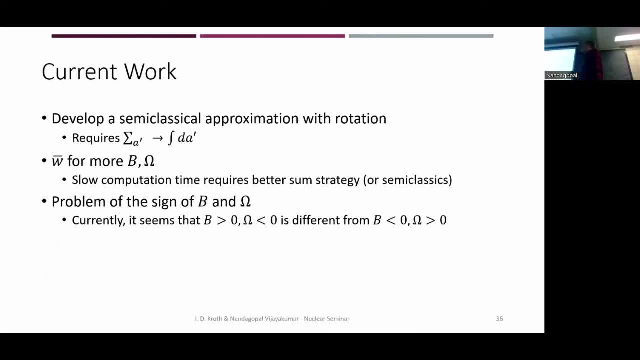 The problem with this is again the slow computation time. We need a better way to sum things, or just do the semi-classics. So- And this last bullet is less of a problem now than it was when I wrote it two weeks ago- 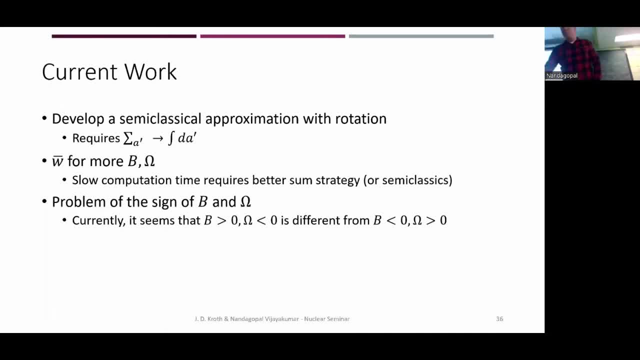 But everything I told you on the last slide may have been slightly wrong, because it seemed without some importantly detailed bookkeeping. it looked like with B pointed this way and omega pointed this way. it was different from having them like this. So essentially, even without rotation, 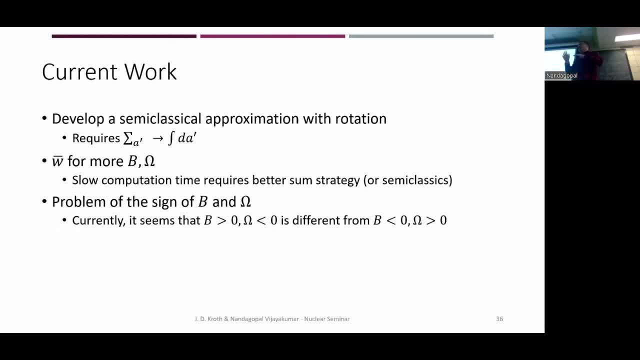 It looked like an electron and a positron in the same magnetic field would be radiating slightly differently, which doesn't seem like it would happen. And likewise, if you had B like this and omega like this, it looked like it was different than this guy. 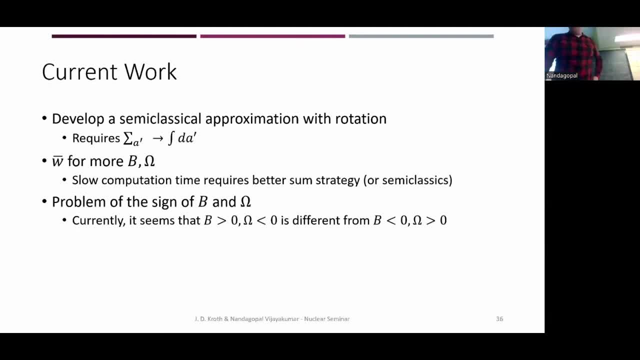 Some kind of charge or parity violating effect. But we think now, since I wrote this, that if we do the detailed bookkeeping and do everything correctly, that doesn't happen and it's all good. We only have two cases of aligned and anti-aligned. 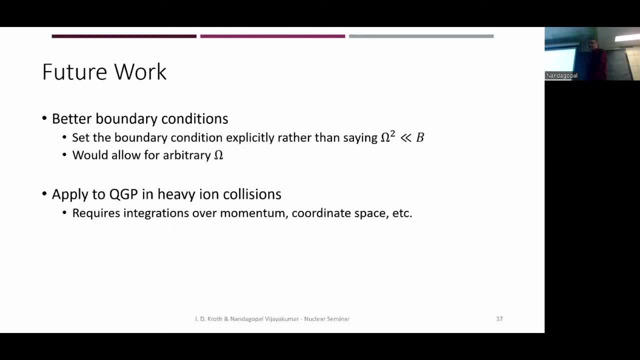 And that leads into the future work that we're looking at. We want better boundary conditions. This is something, actually, that Dr Pizzeggoli and Dr Duchin are working on now, But we said omega squared, essentially, is much less than B. 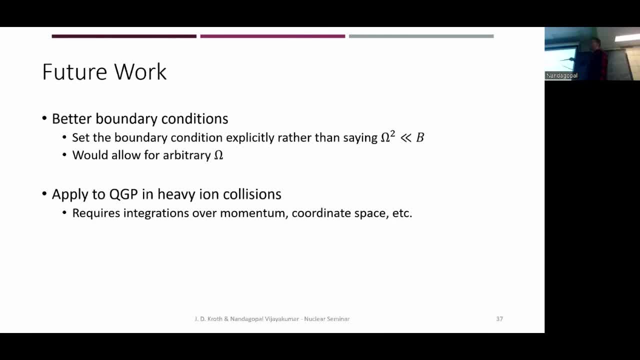 We want to say: what if omega squared is less than B? What if omega squared is much greater than B? What if it's about the same as B? Because then we have arbitrary omega and we can do more predictions, At least when I saw it essentially in our I functions way back when. 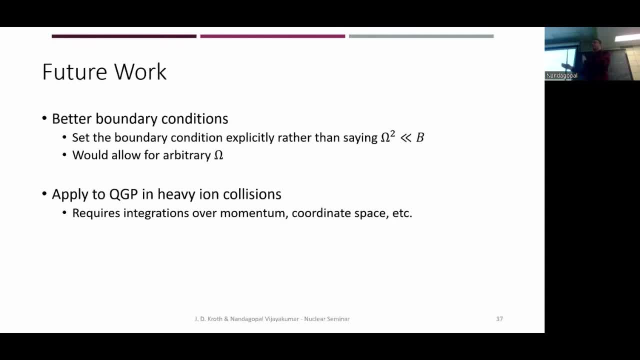 we had those Laguerre polynomials, Those essentially changed to hypergeometric functions, which are famously hard to converge. And then our n values: instead of being integers, they become real numbers that correspond to zeros of the hypergeometric functions. 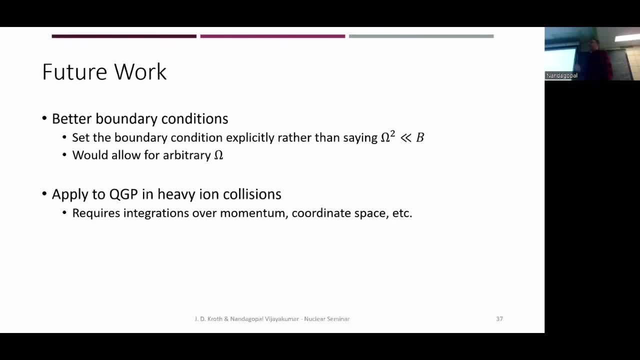 We need to renormalize our wave functions so that it's an incomplete integral over hypergeometric functions. There's got to be a better way And essentially all that comes from setting the wave function, or rather the current, the radial component of the current. 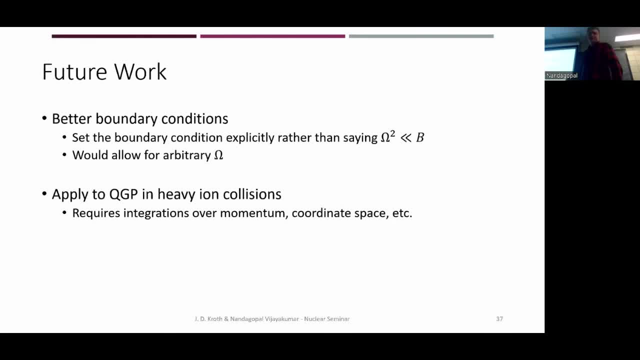 equal to zero and just getting all that out, And then eventually the nuclear physics approach. we want to look at core-coulomb plasma and heavy ion collisions. To do that we need to get from one fermion to many fermions. 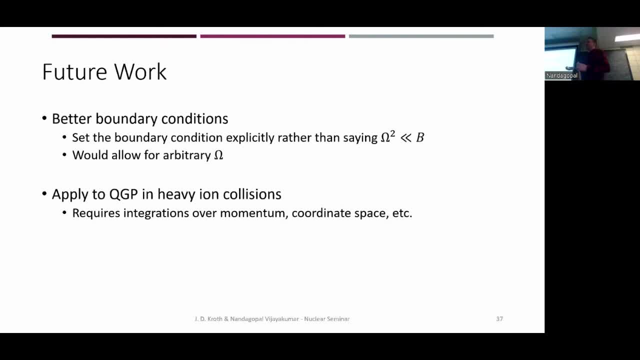 which means integrating over the momentum space, integrating over the coordinate space of the plasma and doing many more computations with the magnetic field as well, And so that concludes the regular part of the talk. There are a few extra slides though, if anyone is interested. 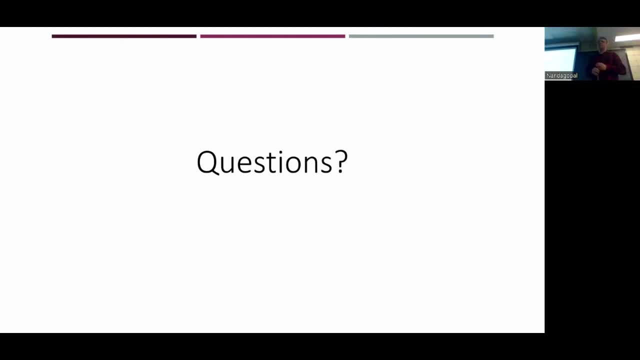 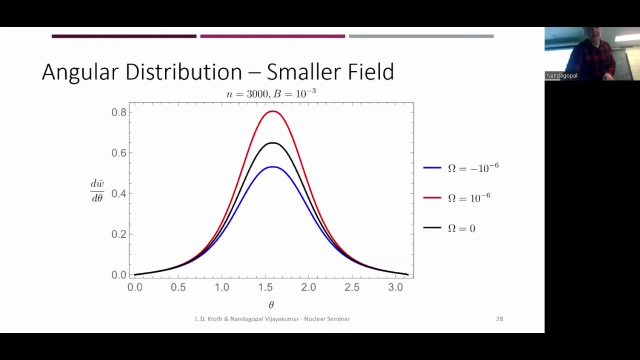 Is there any questions for the audience here? Yep, So we choose which terms to calculate. in sum, by looking at, You find a peak at a particular theta. right Yeah, We go to essentially pi over 2 where this guy lives. So you have this rotation-less expectation. 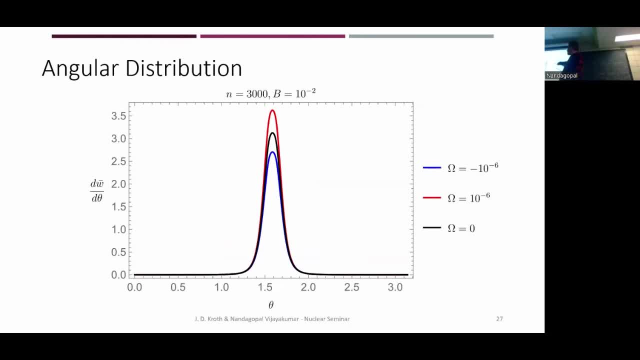 or, as a result, the black curve is from no rotation, right, Right, So you expect there to be a peak there? Do you worry that you've biased the computation at all by starting like only looking at this theta value and not doing a scan of like symmetric flows? 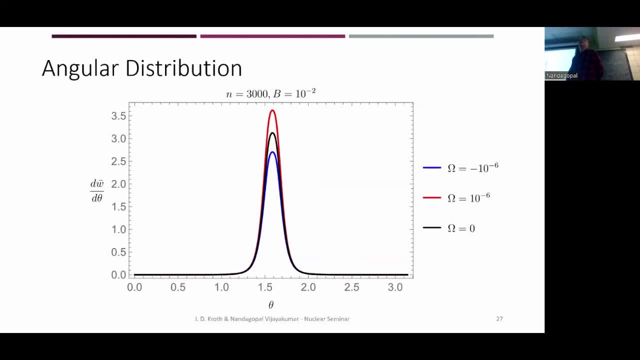 Right. There is, I do recall at least one computation where I think lower magnetic fields tends to spread this out. Lower magnetic fields and higher energy tends to spread this out a little bit, But so far it doesn't look like that's occurring. 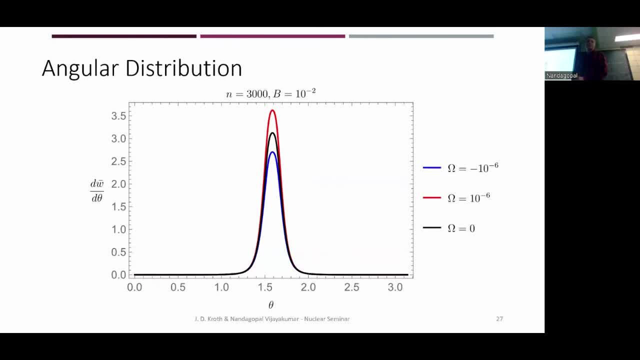 Essentially just need to look at it- more data, more cases- But it seems like a pretty good strategy so far. So this thing always has a peak in the middle, Yeah, And even if it isn't sharply peaked like this, it's, you know, more softly peaked. 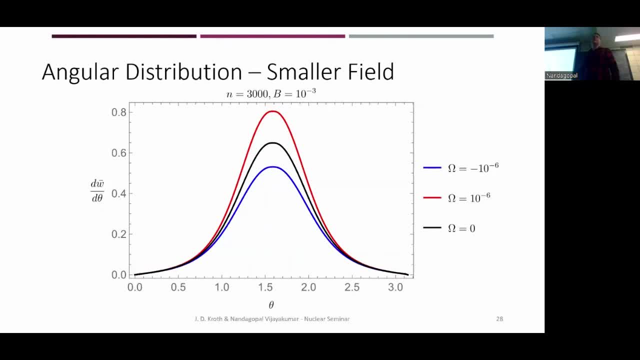 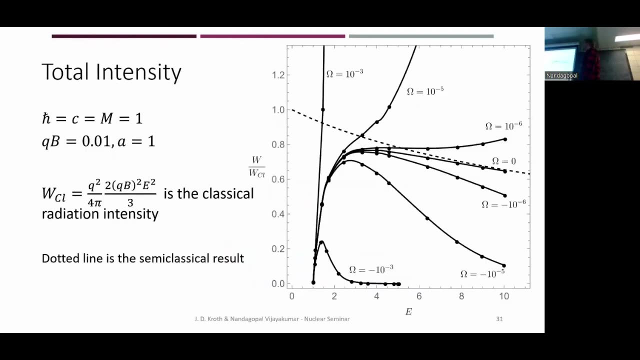 So it's a good indication and indicator of how we do things, of how the slump is going. Yeah, Can you go forward a few slides? Okay, Yeah, So did you mention why? Did you know why some of this almost exponentially starts to increase? 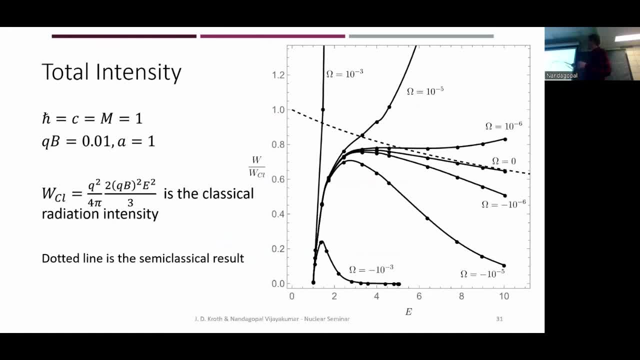 when this omega becomes small Becomes. Well, when omega there decreases, right, It's almost like No, it increases. sorry, Yeah, Not particularly, It's kind of just. It comes out of the numerical approximates that way. 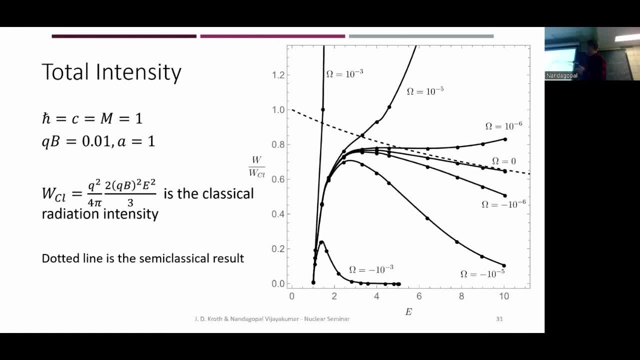 I mean, if you stare at this, if you plot essentially the ratios of these, like this curve to this curve and this curve to this curve, they follow roughly the same line, which is about exponential, But if it's, Or it looks exponential, 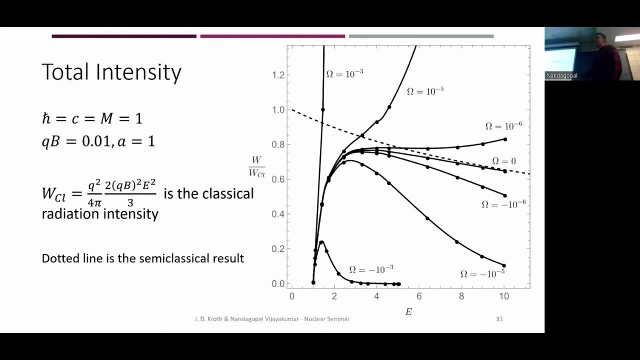 but anything concave up looks exponential. but So I mean, if you were to guess, if you just keep increasing this, do you think it will still increase exponentially? That would be. I don't think so, Based on at least this guy. 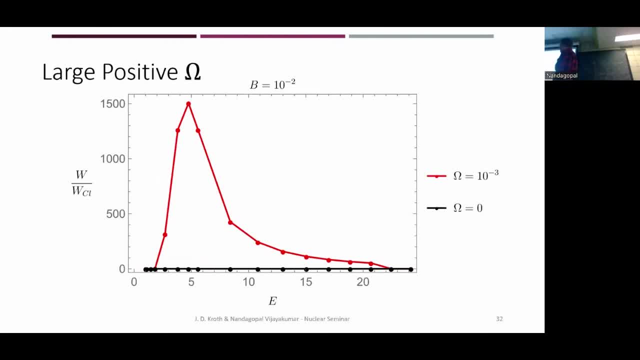 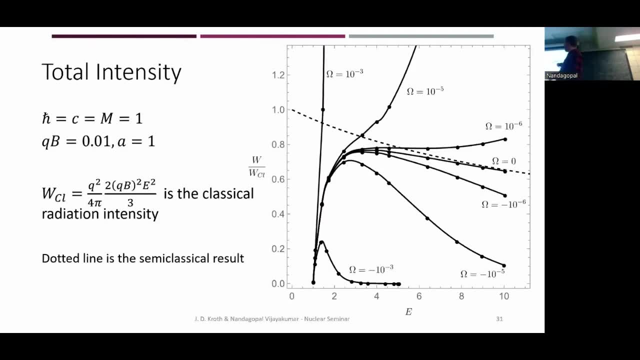 you know it shoots up, but then it starts to come down almost exponentially. Just eyeballing it, Yeah, but I mean the peak though Of right here, Right, I mean the peak of every curve, right, Right, If you keep increasing omega. 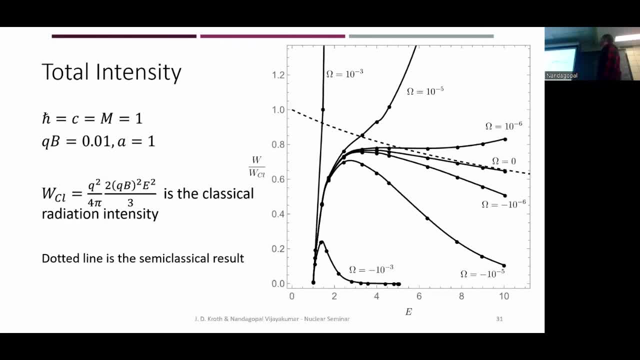 will it still keep increasing exponentially the peak? That's a good question. We haven't gone much higher than this because we're running off against B there, But it's something to look into And we could do it the other way as well. 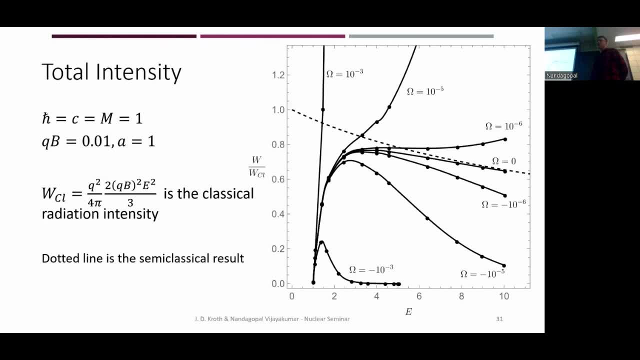 continuing to get suppressed like that, Right, So It looks like the. It's really like this. Can you, Is it possible, like to match this curve? Is it the same shape It's is? Yeah, I think so. 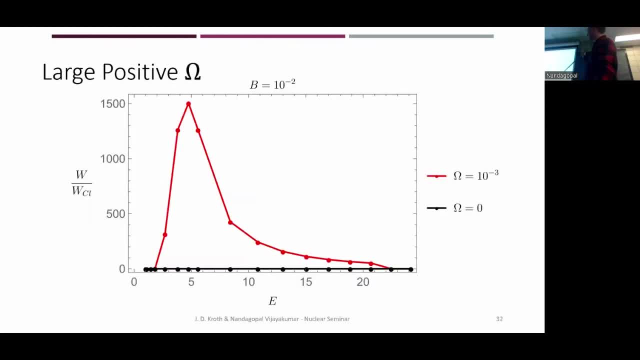 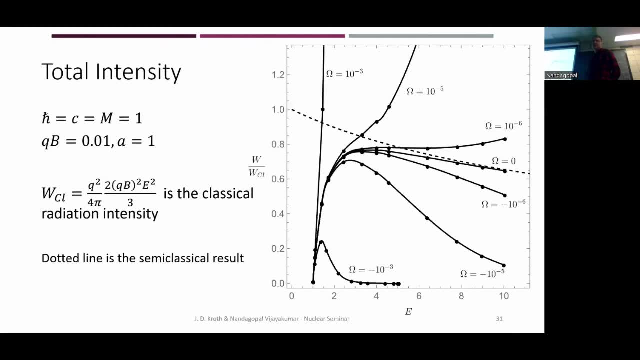 Roughly. I mean, you know, I think you know, I just showed this next slide. you know, if you scale this down, would it match this minus? Potentially? That's again something to look at Roughly, like I just said, roughly. 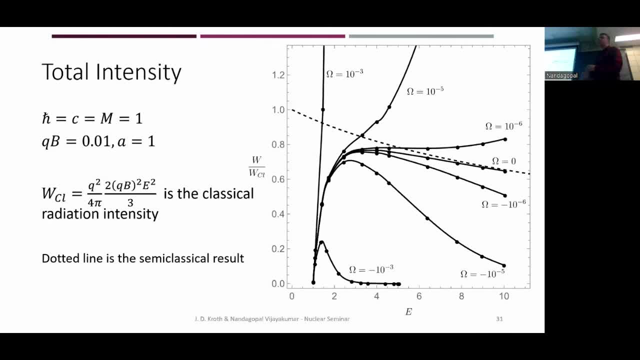 the ratios of these guys to the non-rocating case do follow the same path, even though they aren't exactly the same. but yeah, It's an open question. is the answer. Yeah, I haven't applied any fitting functions to it yet, but 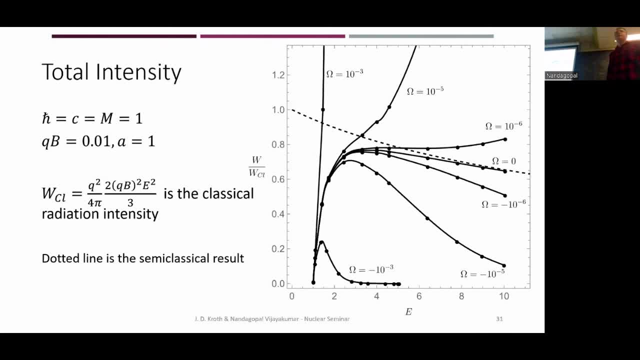 No, I mean like just once. Oh sure, I haven't done anything with that yet, but it's a good suggestion, Yeah, Yeah. so I mean, at the end, the goal is to apply these two. 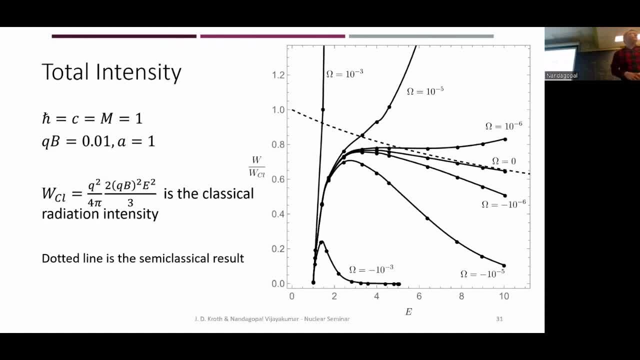 So geometry now is: you're assuming that you have a cylinder right, Right. So even before going beyond that, can we ask how complicated would it be to do a little further by implementing this football shape at the QEG plasma hat when it starts rotating? 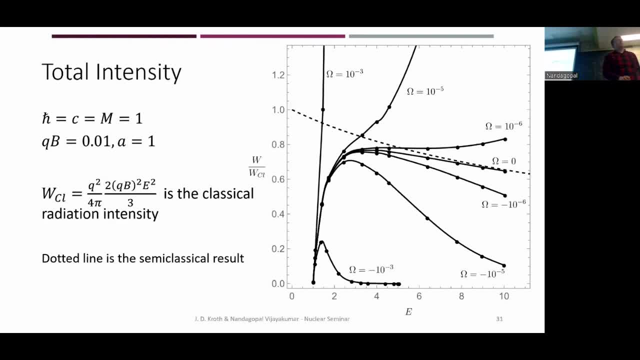 I mean in a simplest way, right, Because this is just. you are assuming this, Right, Assuming the curve, just assuming that, Yeah, That's very close. Yeah, That's not something that I'm very knowledgeable about, but I imagine, if I'm 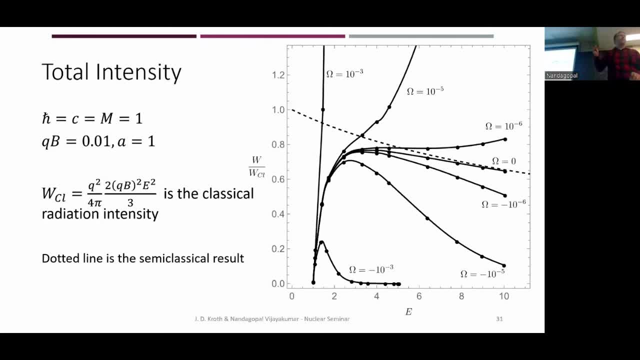 just imagining this in a very simple model. we could just say we have many of these identical fermions with a locally constant magnetic field and then just integrate over some density function in position space, Exactly, And it's just, you know. I feel like it's a very good idea. 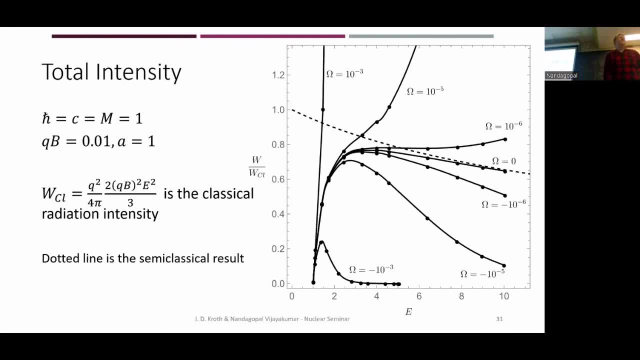 This is like my first naive order model or zeroth order model. Is there any questions from the Vocal Studio? Yeah, just a clarification. like what exactly did like the A's and the A primes refer to? A and A prime were those quantum numbers we had closer to the beginning? 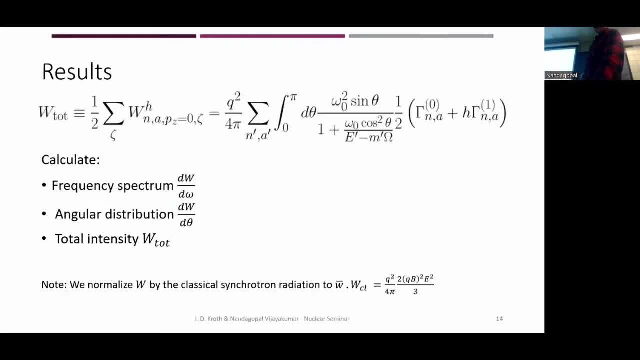 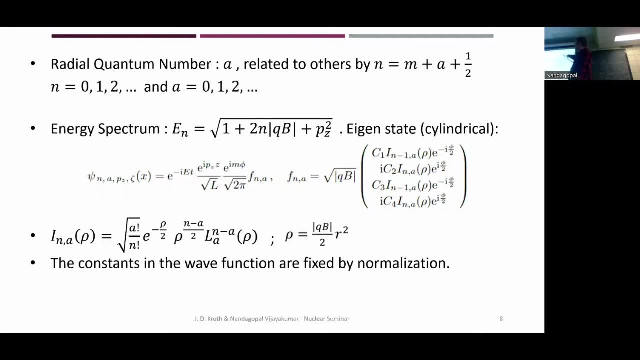 Essentially it's true of the like. we're going to try to get out of this a little bit quicker, right? Yeah, essentially just related to this n and m, the angular momentum number, the principal number, just a way to rescale things.